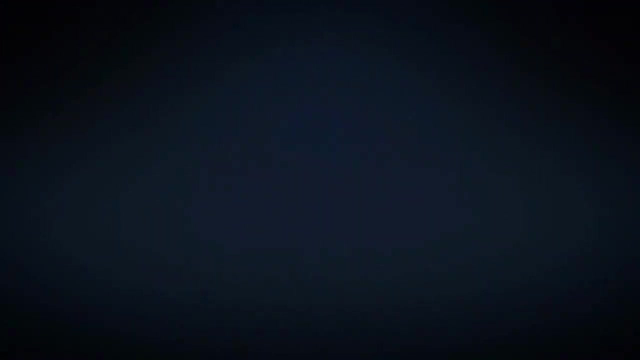 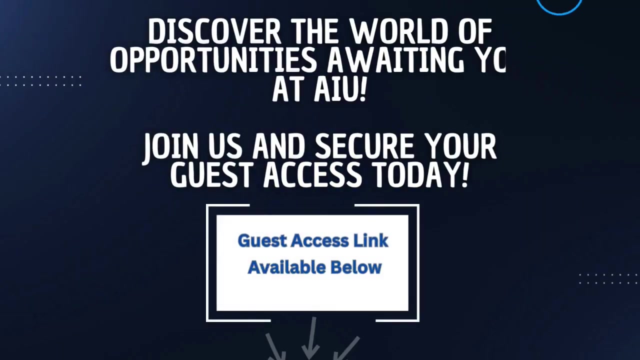 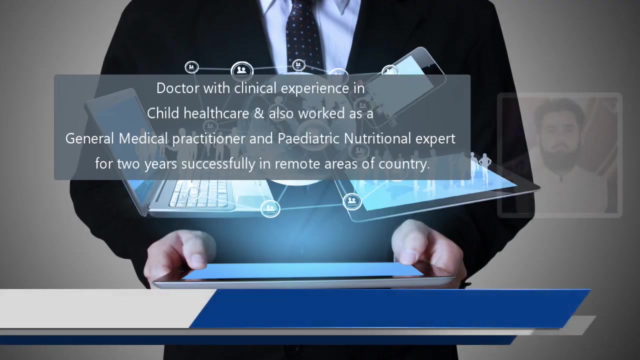 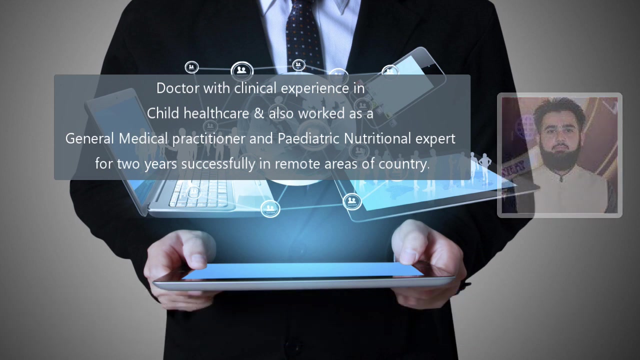 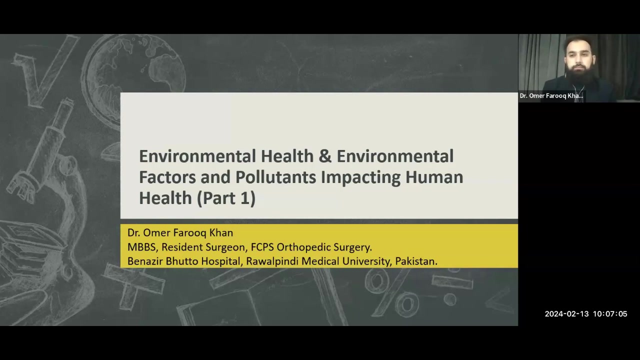 Okay, so our next topic of presentation is environmental health, which is a very broad and very important subject, especially in this century of ours, as we are already witnessing climate crisis and all So environmental health and environmental factors and pollutants impacting human health. So this is part one of our lecture. Basically, this is a lecture series. 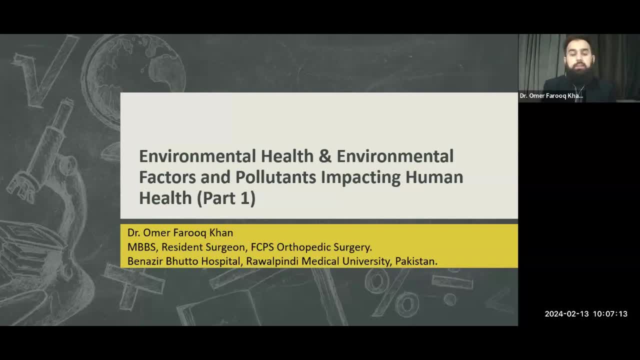 and this is a very wide and very diverse subject So it would be unwise and unjustified to just touch it and do not go into the basic details and do not go into the specifics And just it will not do justice if I try to cover it in one sitting. So I will try my best to deliver the 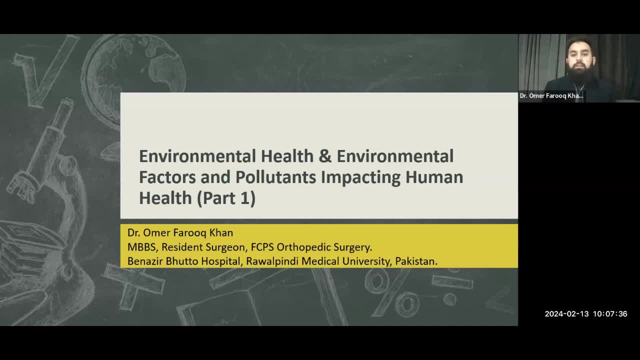 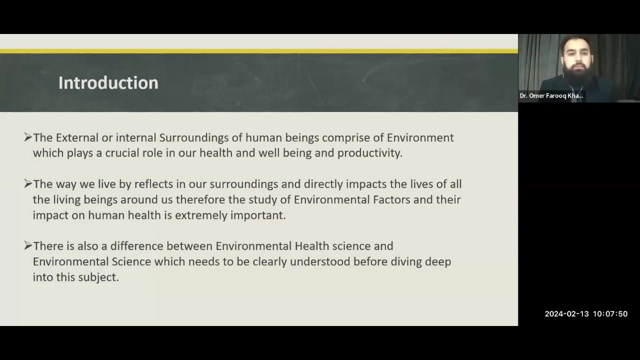 basic definitions and basic concepts about the environmental health and then we'll move on to the environmental factors and pollutants impacting human health. So, introduction: The external or internal surroundings of human beings comprise of environment, which plays a crucial role in our health and well being and productivity. The way we live by reflects in our surroundings, and directly. 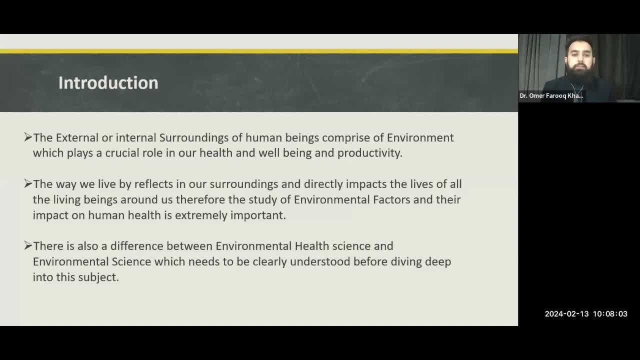 impact the lives of all the human, all living beings around us. Therefore, the study of environmental factors and their impact on human health is extremely important. So the way we live by is basically what we choose our environment to look like. If we have a very healthy lifestyle, 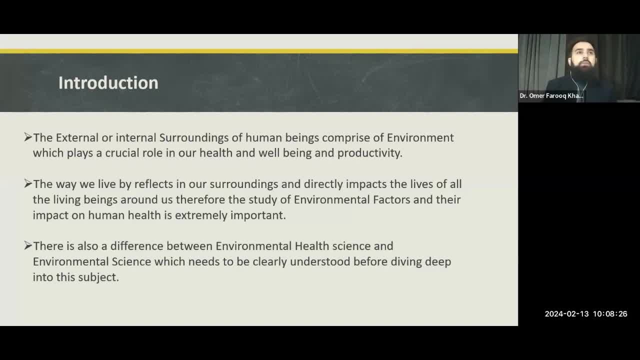 if we care about our external environment, if we care about the place where we live in, if we care about the people we live with and if we care about the animals and plants and all the living things we live with, then the environment we are living in will be a beautiful environment. 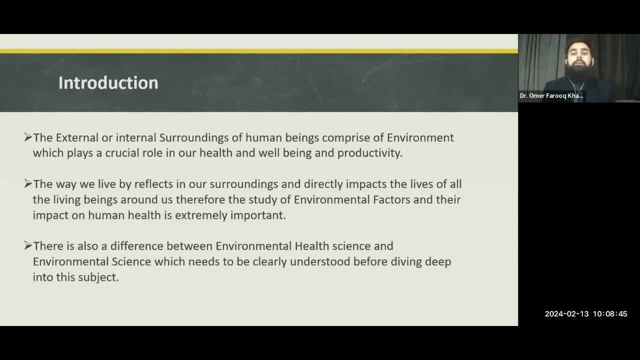 And if we do not care about our environment, then definitely our environment will start to get deteriorated due to human activity and therefore the way we live by reflects in our surroundings and directly impacts the lives of all the living beings. It's not just humans. I never I didn't write human beings. I'm writing the living. 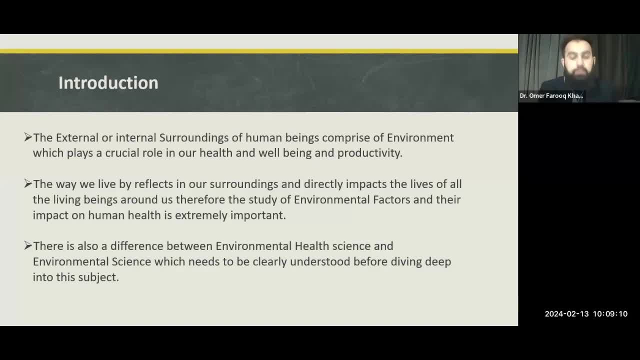 beings around us. Therefore, the study of environmental factors and their impact on human health is extremely important. There's also a difference between environmental health science and environmental science, which needs to be clearly understood before diving deep into the subject. So there is a clear difference between these two. 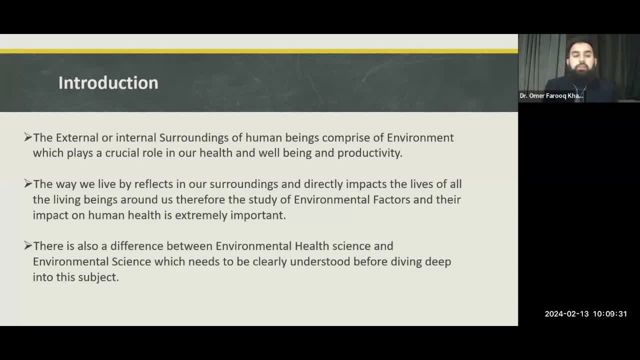 sciences. One is the study of environmental things like environmental sciences. It is a very broad term. Environmental sciences covers almost all of the basic life sciences and physical sciences as well, And there is an environmental health science. What's the difference between environmental health science and the environmental sciences? We will cover it ahead. 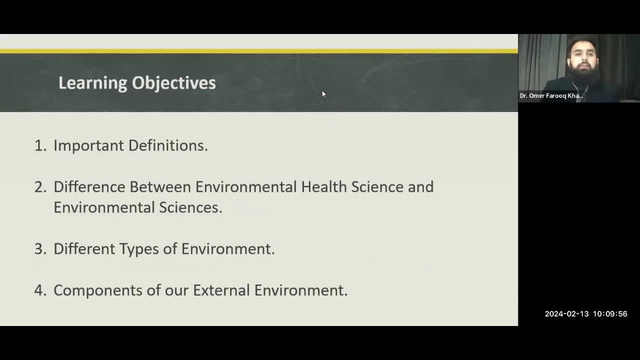 So the learning objectives for our class First of all. as is the style of my teaching, I always start with the definitions. So the learning objectives for the class of environmental health is important definitions. So first of all, we will try to understand what we are going to talk about in our today's class. So important definitions. 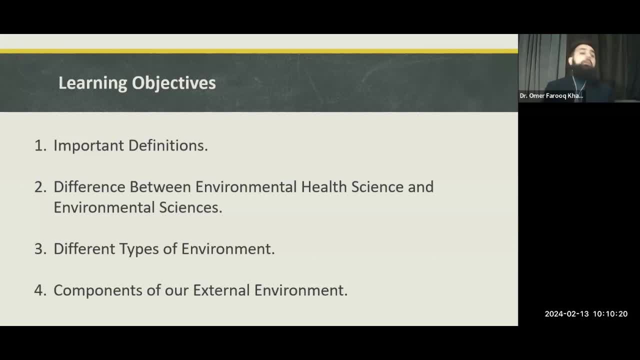 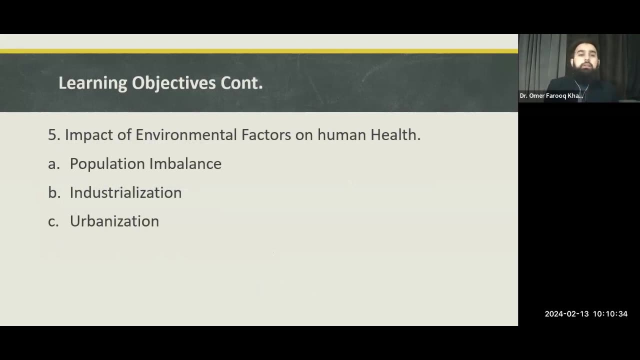 Then the difference between environmental health science and environmental sciences, Then different types of environment, Then components of our external environment, Then impact environmental factors on human health. There are many factors which impact human health, Many environmental factors which impact human health. But as it is a very broad and very wide, 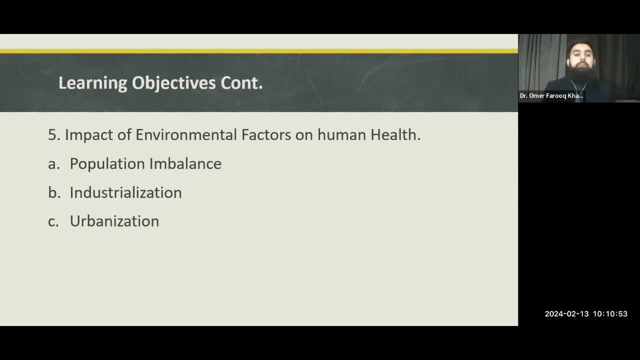 ranging subject, So I will cover three. So there are three basic environmental factors in today's class. One of them is population imbalance. Look, I did not write population explosion, because this is a misnomer these days. So I wrote population imbalance And I will justify why I did not write population explosion. basically. 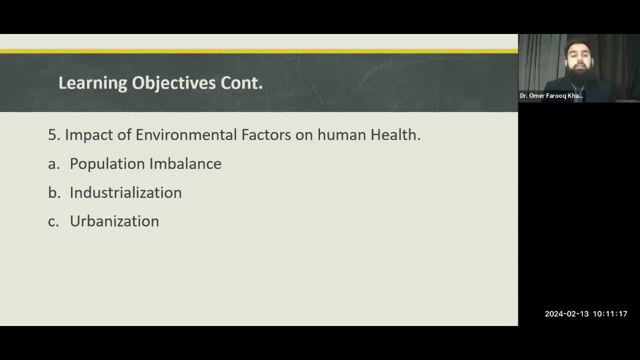 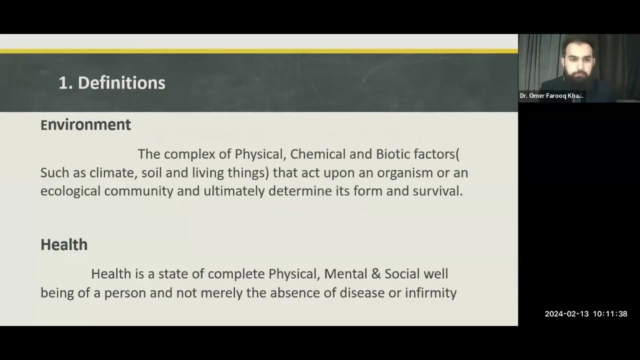 Then there is industrialization. The second environmental factor impacting human health is, And then there is a third subject which is affecting human health, that is urbanization. So we'll start with important definitions. So number one definition is: what is environment? So all of you people must be thinking that we are starting to understand what is environmental health. 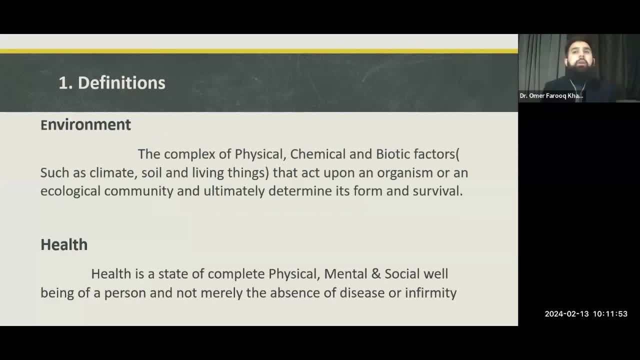 But without a basic understanding of what environment is, we cannot go ahead and talk about the environmental health. So what is environment? Environment is the complex of physical, chemical and biodefactors, such as climate, soil and living things, that act upon an organism or an ecological community and ultimately determine its form and survival. 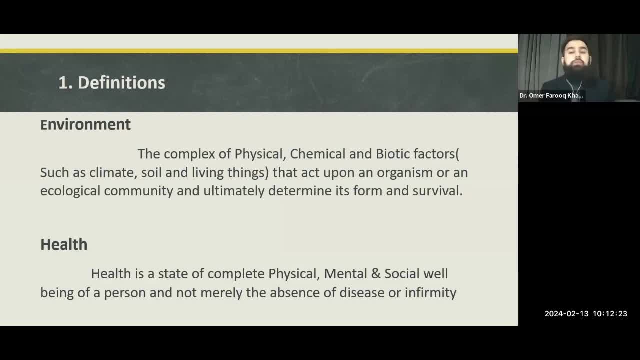 So any complex of physical, chemical and biodefactors which act upon an organism or which form the surrounding of an organism or any ecological community and then ultimately determine its form and survival is basically an environment. And what is health? We already know what is health. 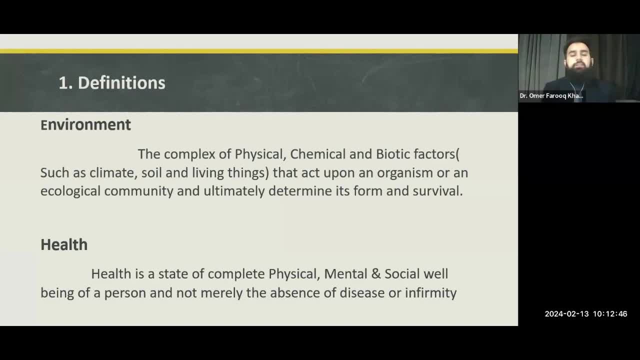 But as we are again and again discussing health-related subjects, so I Cannot emphasize enough the basic definition of health. So health is a state of complete physical, mental and social well-being. Always remember it's not just physical and mental. 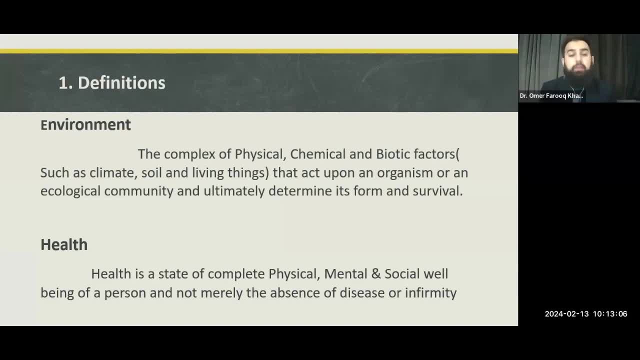 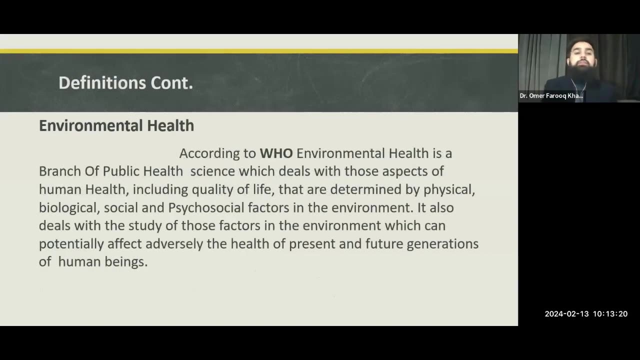 It's social well-being as well. So health is a state of complete physical, mental and social well-being of a person, and not merely the absence of disease or infirmity. Then there is a definition, The definition of environmental health. So there are many definitions of environmental health sciences. 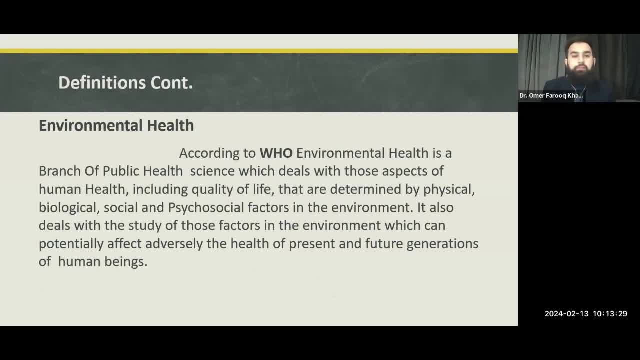 So I chose the WHO- World Health Organization- definition. So, according to WHO, environmental health is a branch of public health science. There are many branches of public health sciences, As I am teaching you people public health-related subjects, So environmental health is also a branch of public health science which deals with those aspects of human health. 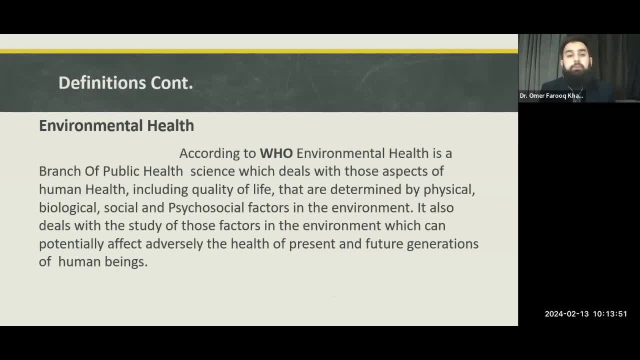 including quality of life, That are determined by physical, biological, social and psychosocial factor in the environment. It also deals with the study of those factors in the environment Which can potentially affect adversely the health of present and future generations of human beings. 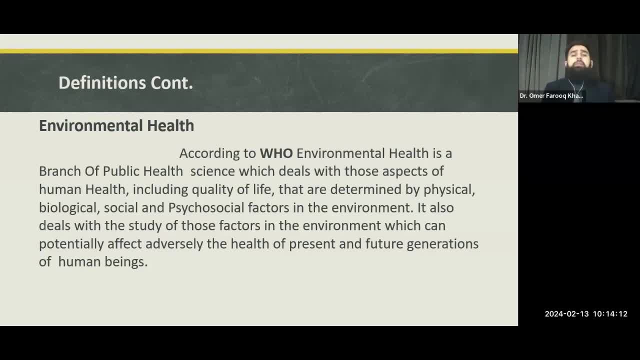 So, basically, The branch of public health science will deal with those aspects of human health, including quality of life of human being, That are determined by the physical, biological, social and psychosocial factors in the environment: by physical, biological, social and psychosocial factors in the environment. 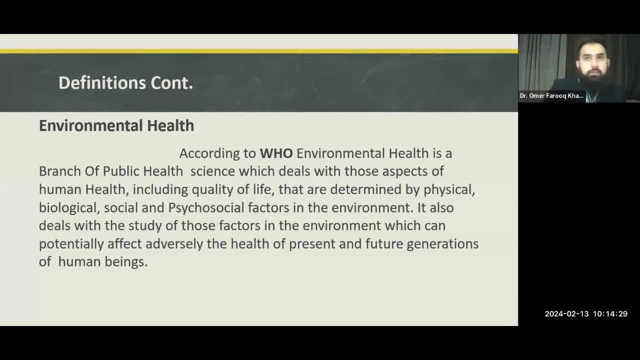 So what the environmental factors have any kind of impact on human health, that is to study this aspect of public health. science is environmental health science. So if a person is living in a bad environment and we start to study the impact of that bad environment on that person's health, 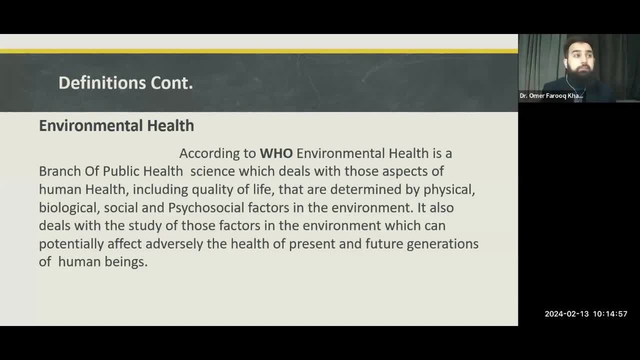 then that aspect will be environmental health related to that person. only If we start taking this to a wider level and we start talking about whole of the human beings- human being species, Homo sapiens species- then this will become a wide-ranging environmental health science. 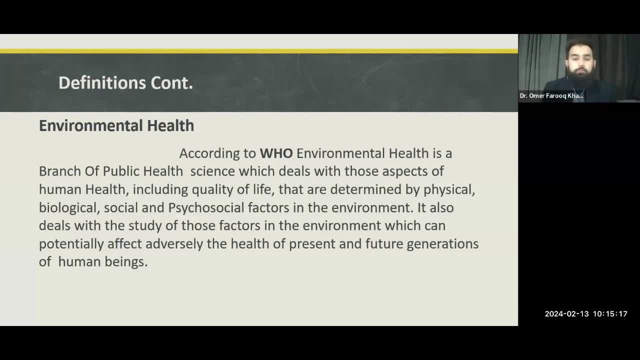 where we will be able to study the impact of that bad environment on that person's health. The environmental factors impact on human health is being studied. So environmental health is a branch of public health science which deals with those aspects of human health, including quality of life. 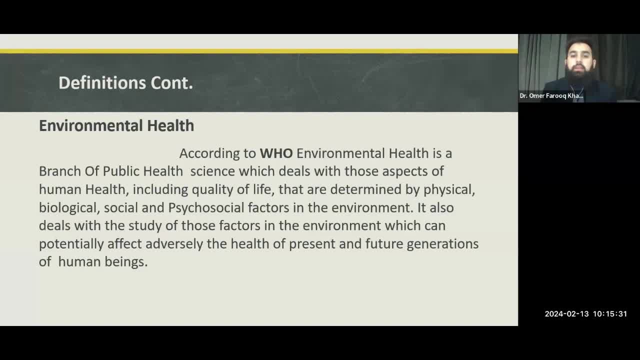 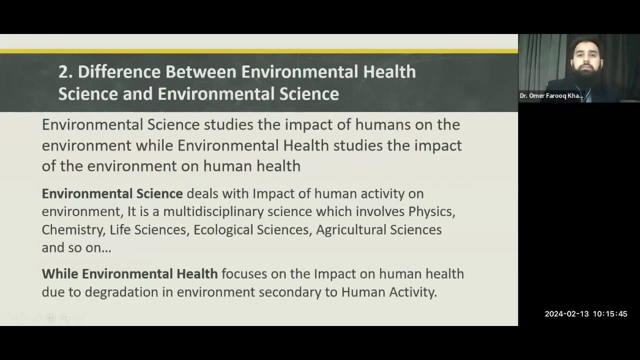 that are determined by physical, biological, social and psychosocial factors in the environment, And then it also deals with the study of those factors in the environment which can potentially affect adversely the health of present and future generation of human beings. Then there needs to be a clear understanding. 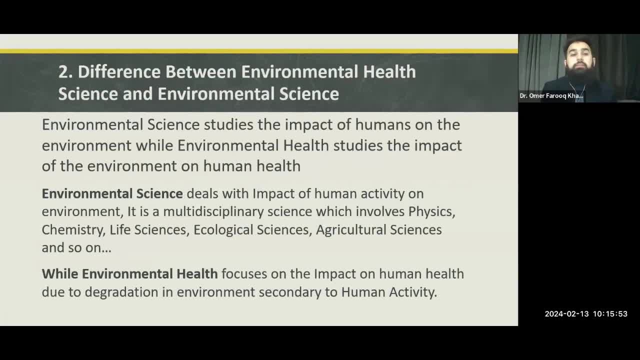 So I took my time and then I wrote about this Difference between environmental health science and environmental science. So basically, if we talk about environmental science, then that is a whole different story, And if we talk about environmental health science, that is a completely different thing. 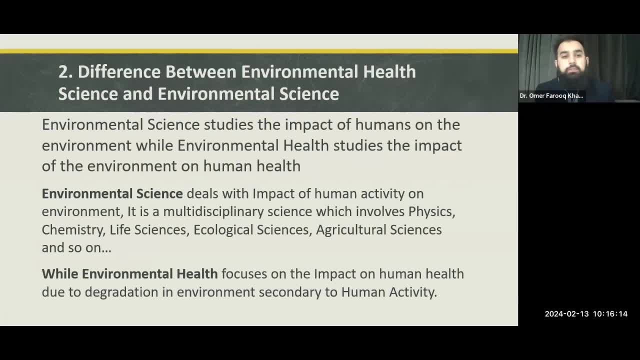 Environmental science studies the impact of humans on the environment. Environmental science studies the impact of humans on the environment. So whenever we talk about environmental science, we are studying the impact of humans on the environment, While environmental health studies the impact of environment on human health. 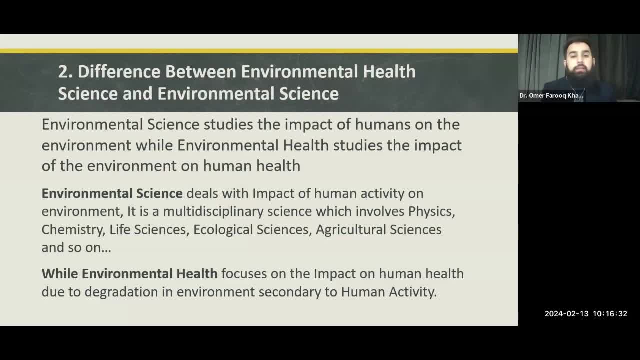 So if we are talking about just environmental sciences, we are studying the impact of human activity on their surrounding environment, And when we are talking about environmental health science, then we are coming to the point where it is only 80 degrees better. We study the impact of environment on human health. 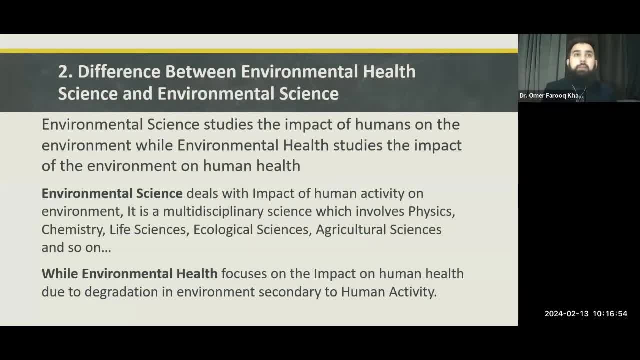 Even if the environment is created by human beings themselves, then that newly created environment, whatever its effect is on human health, that will be studied in environmental health science. Environmental science deals with the impact of human activity on environment. It is a multidisciplinary science which involved physics. 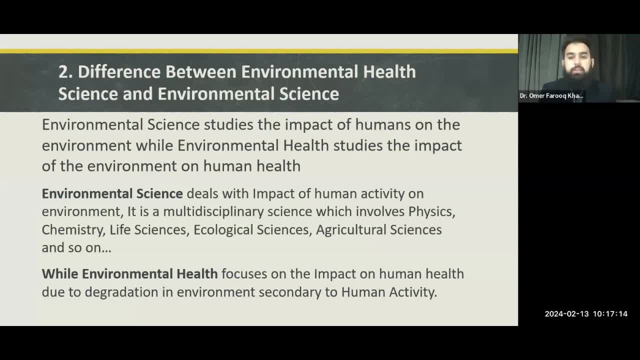 chemistry, life sciences, ecological sciences, agroecology- So it has an impact on the environment and the environment itself, cultural sciences and so on. So environmental sciences are also a broad thing, It's not just a single science. Any physical or life science that we study comes under the umbrella of. 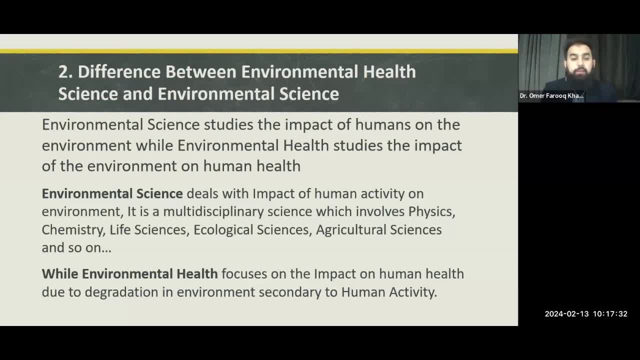 environmental sciences, While at the same time, when we talk about environmental health science, environmental health focuses on the impact on human health due to degradation in environment secondary to human activity. Mostly, it's just like that. Then I just added some images Then. 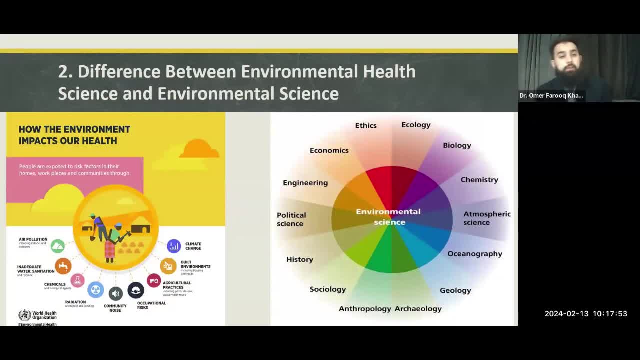 there is a World Health Organization image about the environmental health, So we just on the left side of the slide how the environment impacts our health. People are exposed to risk factors in their homes, workplaces or communities through air pollution, inadequate water, sanitation. 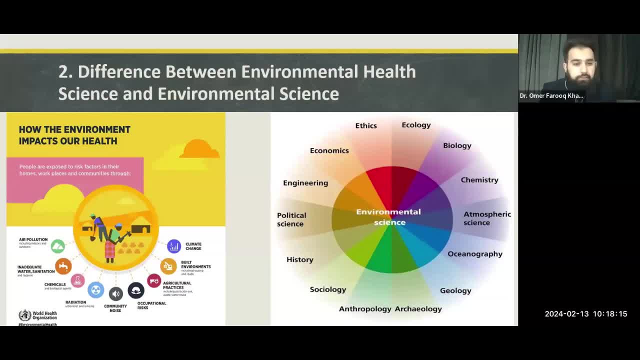 chemicals and biological agents, radiation, community noise, occupational hazards. Then there are agricultural hazards or agricultural practices, including excessive use of pesticides, et cetera. Then there is built environment hazards. Then there is the climate change. So whatever harm we created in our external or internal environment, and then we have a threat to it, then what we do is we destroy it. So we have to歌, and then we have to ikii, and we just destroy it, Because if we compens't for it, if we don't, So, whatever harm we created in our external or internal environment, and then we have to�이. 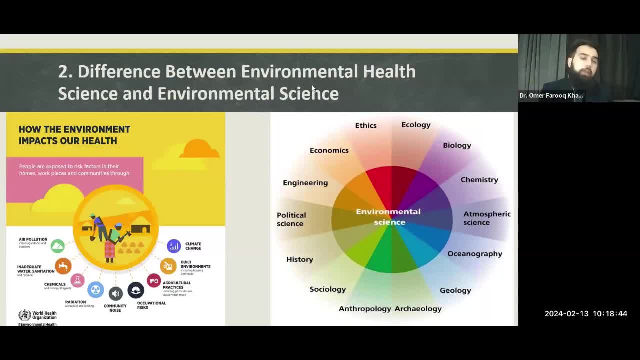 that harm affecting our own health. when we start studying that, then that is environmental health. so whatever the bad environment or unhealthy environment has any kind of impact on human health, that will be studied under the umbrella of environmental health science. so, and similarly, what environmental sciences covers on our right side, environmental science covers many kind of environmental 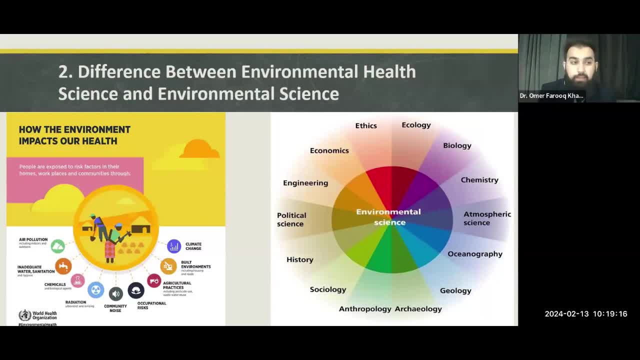 sciences, including social sciences, including life sciences, including physical sciences. so social sciences, just like political science, ethics, economics, these are social sciences- history, sociology, anthropology. and then there are physical sciences such as engineering, chemistry, physics, geology, oceanography. then there is life sciences such as ecology, biology, archaeology, etc. so basically, environmental sciences is also a wider umbrella where we 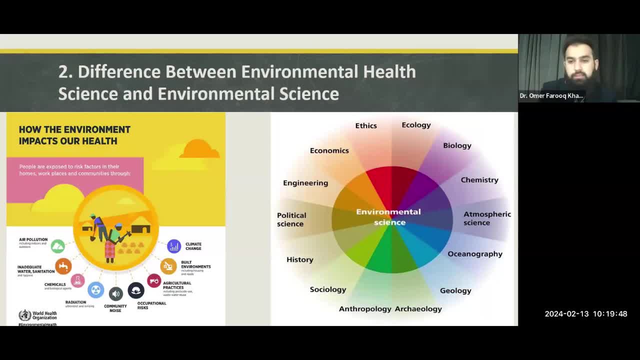 also study social sciences, we also study physical sciences, we also study life sciences. so all of these sciences, uh, come under the umbrella of environmental science, while the environmental health science covers the impact of environmental factors on human health. i hope everyone got this concept clear, because this concept is very, very important when we are moving ahead. 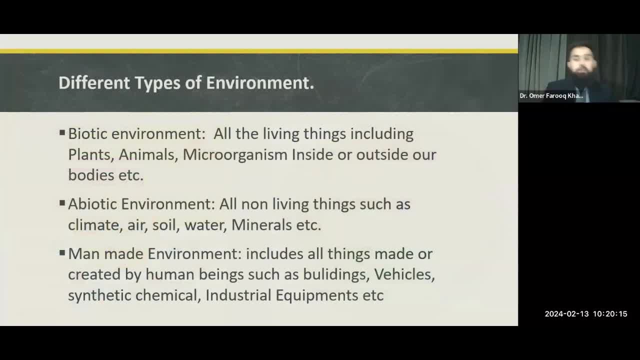 then we start talking about what environment is. now, basically, our actual topic is starting from here. so what actually an environment is? we already talked about that. then there are different types of environment. so whenever we talk about types of environment, there is biotic environment, abiotic environment. 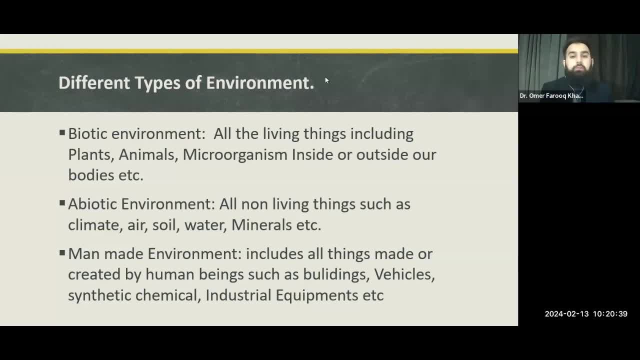 environment and man-made environment. so what is biotic environment? all the living things, including plants, animals, microorganisms, inside or outside our body, etc. whatever living things which we encounter or which have any kind of impact on our environment and in, in the end, on our health due to any kind of change that they bring in our environment. 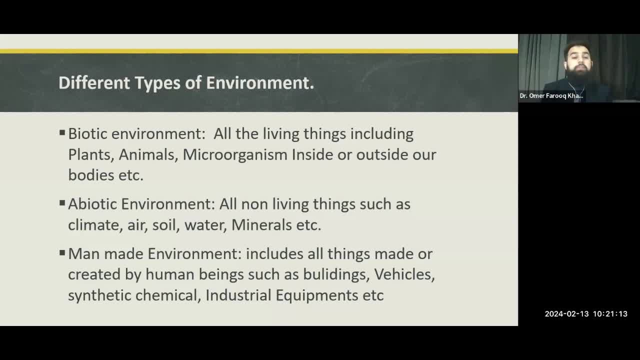 then that is biotic environment. similarly, what is a biotic environment? all the non-living things, such as climate, air, soil, water, mineral, etc. so all the non-living things which are part of our environment and they also impact our life. they also impact our health. 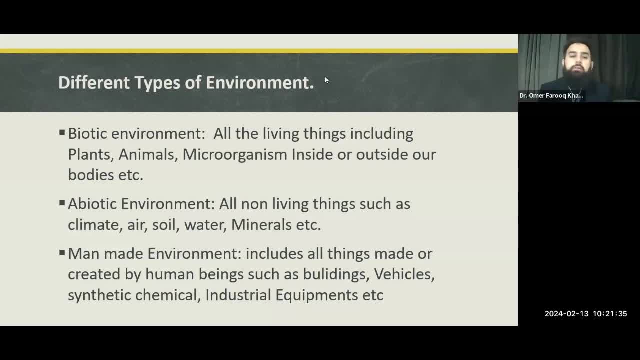 they are part of abiotic environment. so all the non-living things, such as climate, air, soil, water, minerals, extra, they form the abiotic environment. then there is man-made environment, so man-made environment comes under the different umbrella, so including it includes all the things made are created by human beings, such as buildings, vehicles, uh, synthetic chemicals, i'm not talking. 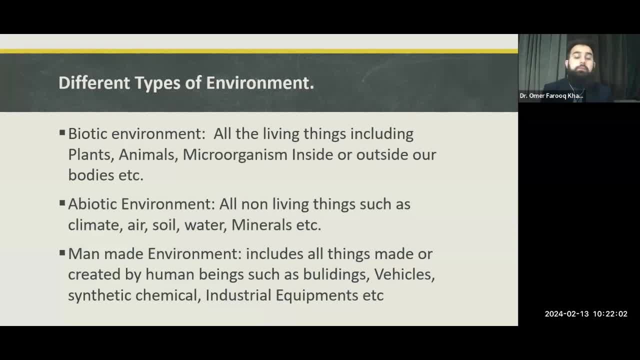 about naturally occurring chemicals, because Naturally occurring chemicals are minerals or organic substances which are naturally occurring. There are synthetic chemicals as well, which are created in our own industries, which are created by human activity. Then there are industrial equipments. So all of this environment which is man-made, it comes under the name of man-made environment. 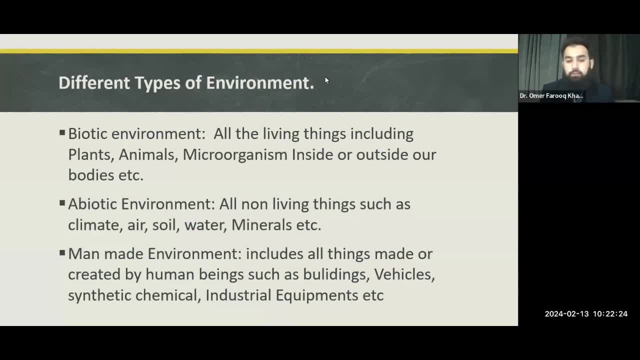 Buildings are not naturally occurring things. Vehicles are not naturally occurring things. Synthetic chemicals are not naturally occurring things. Industrial equipment does not come out of its own. Everything has been created by human beings. So the environment which has been created by human beings- and it also affects our lives, then that is man-made environment. 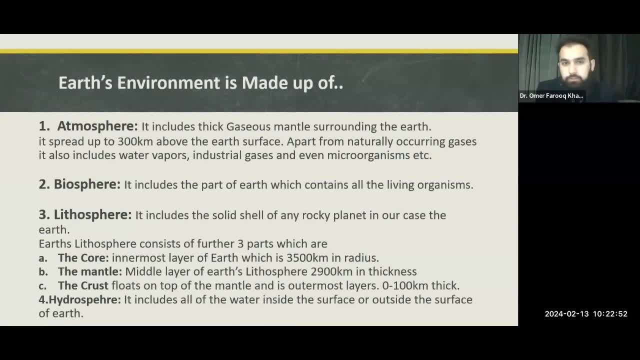 Then Earth's environment. So our planet is Earth, So we will talk about Earth's environment. So Earth's environment is made up of atmosphere, biosphere, lithosphere and hydrosphere. Atmosphere includes thick gaseous mantle surrounding the Earth. 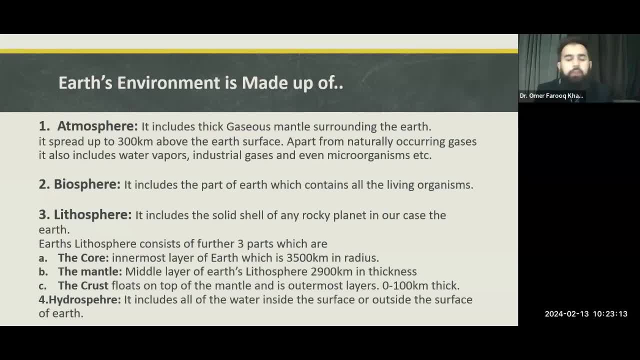 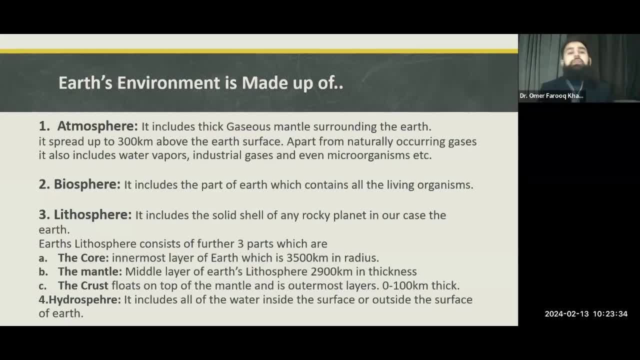 If a rocket takes off. If a rocket takes off from the surface of the Earth and goes beyond 300 kilometers above the Earth's surface, then it clears the atmosphere of the Earth. So the thick gaseous mantle surrounding the Earth forms the atmosphere of the Earth. 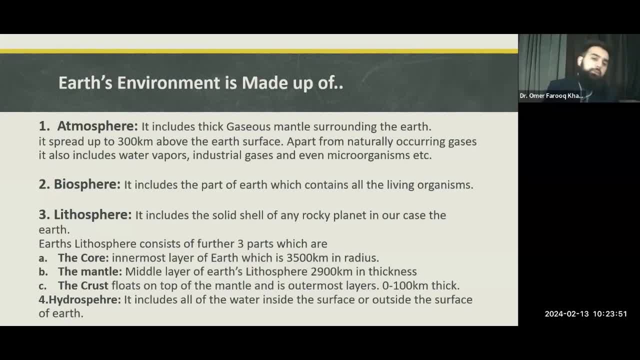 It spreads up to 300 kilometers. Some books write it to 50.. Some books wrote it to 70. Some books wrote it to 300. And some books even wrote it to 320 or 330.. But most of the books say: 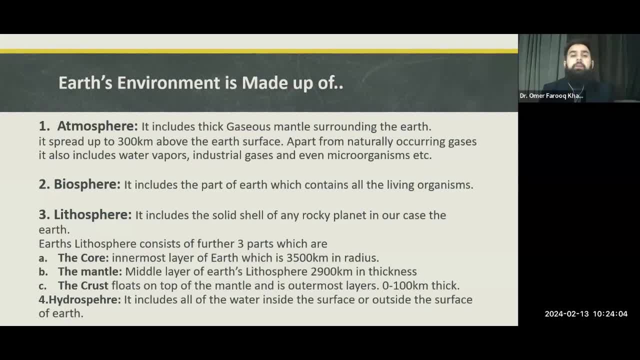 But most of the books say it spreads up to 300 kilometers above the Earth's surface. Apart from naturally occurring gases, it also includes water vapors, industrial gases and even microorganisms. So basically, atmosphere includes of gases. It includes of air. 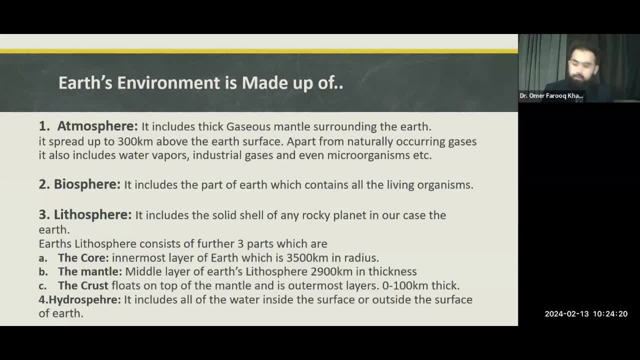 So our atmosphere is made of air. 79% of the air is nitrogen, Then there is almost nearly 21% of the air is oxygen. And then there are many other ways, Other gases as well, Many other substances as well. There are water vapors in lower atmosphere as well. 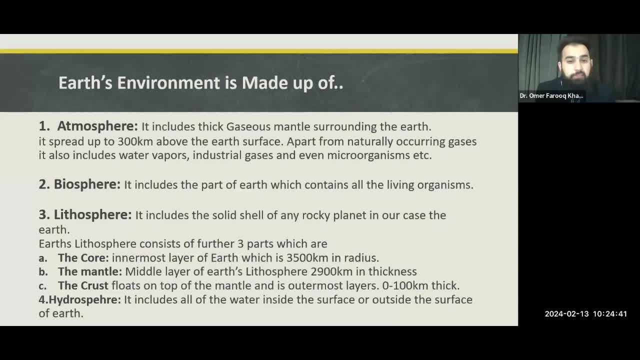 Then there are industrial gases, which have been eliminated over the course of last two to three centuries, are also there And they are not going anywhere. Then there are suspended microorganisms and microparticles as well. All of these things are present in our Earth's current atmosphere. 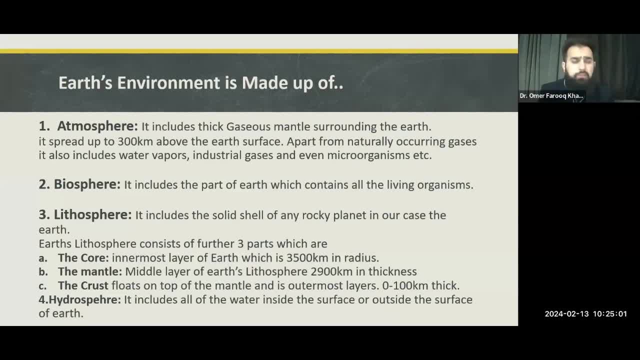 Then there is biosphere. So biosphere, Biosphere means the part of the Earth which contains all the living organisms. So biosphere is the part of the Earth which can sustain, which can create or which can sustain the living organisms. So biosphere means from the depth of the ocean to that part of the atmosphere where microorganisms can stay alive. 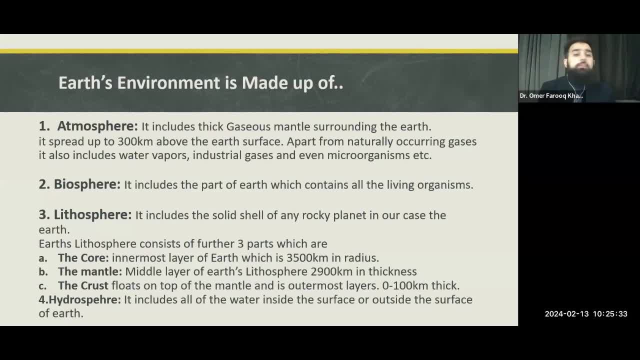 part of the earth which contains all the living organisms is biospheres. it can contain all the deep caves. it can contain all the deep uh oceans. it can be uh high above the sky wherever any living organism. it can be in hot water fountains, it can be around, even around lava. lava even even around. 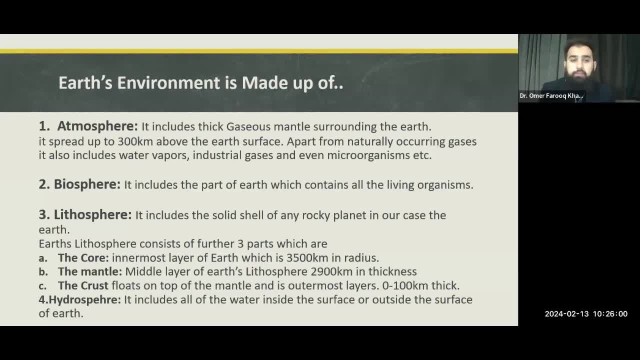 lava, even around hot springs, even around caves, even around and even in the depths of the ocean, even in the at high above uh the art surface, even in the atmosphere. also, wherever there is any kind of living organism, it is biosphere. then there is lithosphere. so lithosphere is uh, includes the 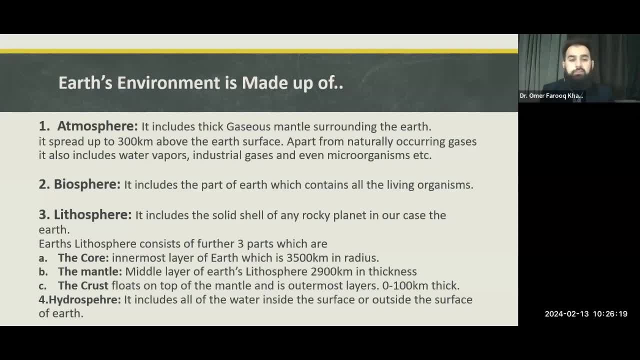 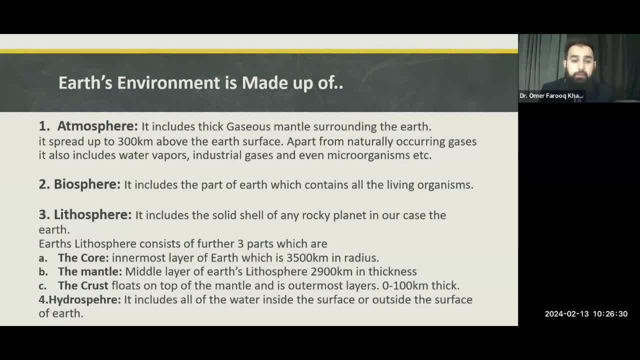 hundred kilometer in radius. then there is the mantle, which is middle layer of Earth's lithosphere, that is 2900 kilometer in thickness. then there is the crust, so the core, the mantle and the crust- the core and the mantle are the vital layers. and then there is crust. crust floats on top of the mantle. 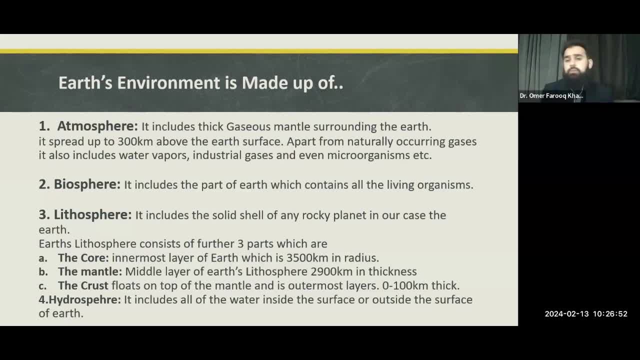 and its outermost layer, and its thickness varies from 0 to 100 kilometers. and then there is hydrosphere. it includes all of the water on the planet Earth, whether it's inside the surface of the planet Earth or outside of the surface of the planet Earth, and hydrosphere include sea water, oceanic. 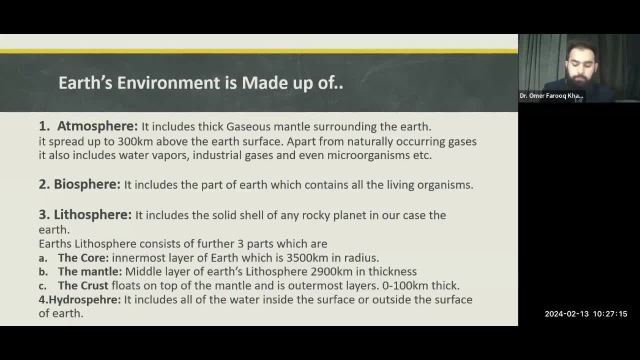 water and fresh water as well. roughly 97 percent of the water, as we already know- most of the people um in in this class would already know that's 97 percent- roughly 97 percent- of the water on the surface are formed by salt water or sea water or oceanic water, and only three percent- 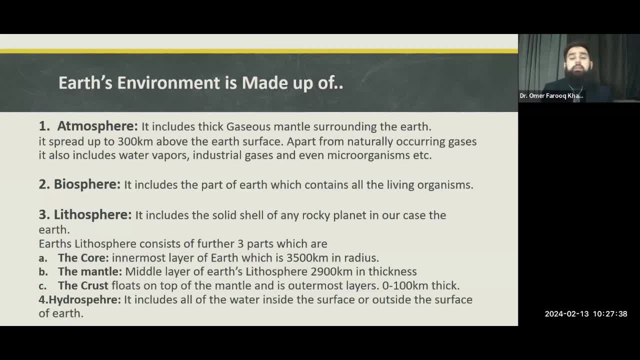 and some books even say two percent of the total water is fresh water. and then the, the fresh water. fresh water is also, you know, divided into the water running in the streams and rivers, etc. and the washed water, water logged up in glaciers, and books say that almost все of this water is from theνη. 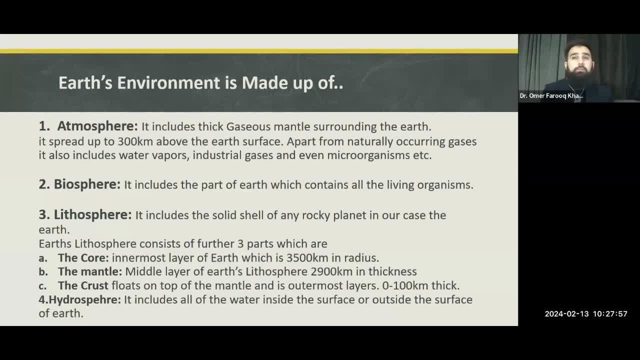 and booksate, that almost in the sea water brown 것을, that almost 65% or 70% of the fresh water is locked up in glaciers and only 35% of the water, fresh water, is running in streams or rivers and underground water, etc. so all of the, all of these spheres, all of these and parts of the 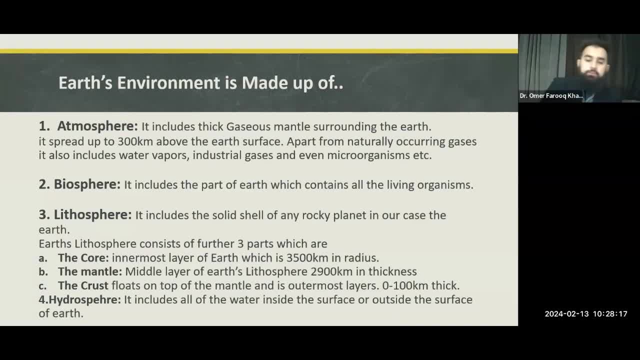 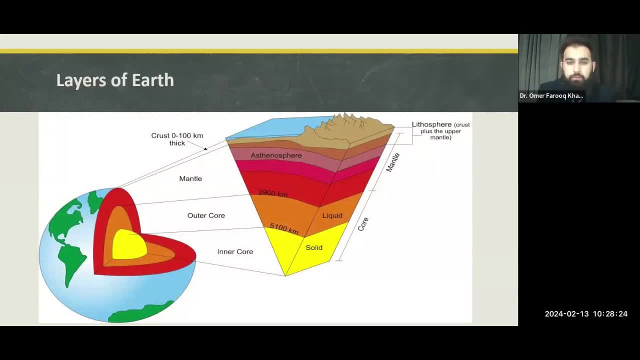 spheres make up the Earth's environment. then there is a diagram about the layers of the earth. we already talked about the core, and the core is roughly 3500 kilometer in radius. the inner, more in the innermost, component of the core is solid, then there is liquid, then there is mantle, and then then mantle and then. 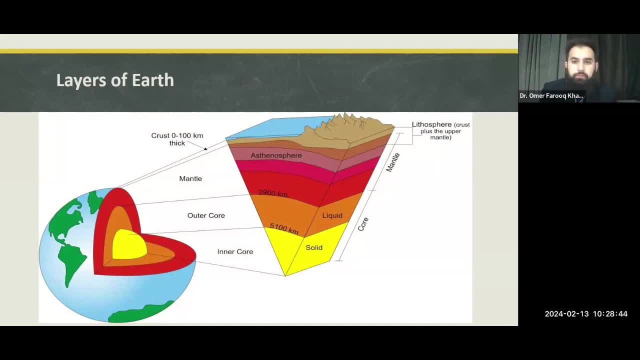 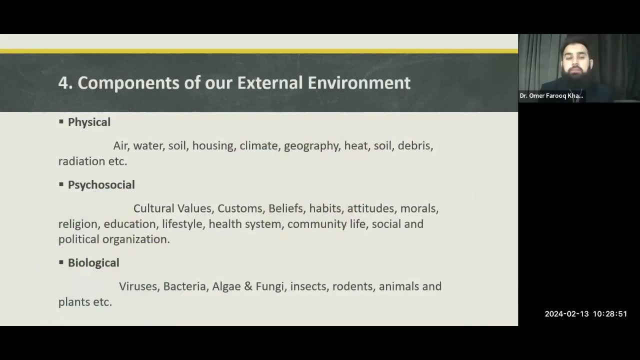 there is crust, and crust is either 200 kilometer in thickness. so then there are components, components of our external environment. so whenever we talk about our human beings, for example, if we talk about our environment, then there are different components of our external environment, and these components are physical component. 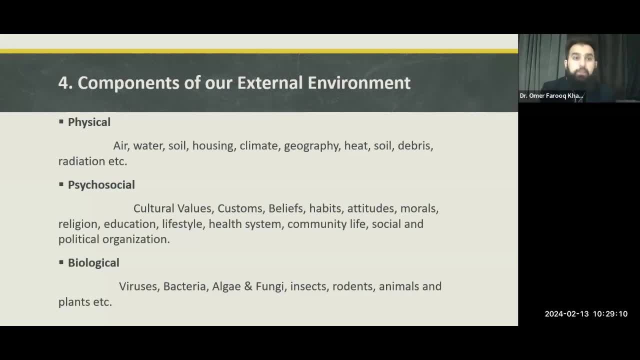 psychosocial component and biological components. so what are the physical component? physical components our external environment are air, water, soil, housing, climate, geography, heat, soil, debris, radiation. so physical components can be a biotic or man-made. so whatever the physical component is, whether it's a man-made physical component, 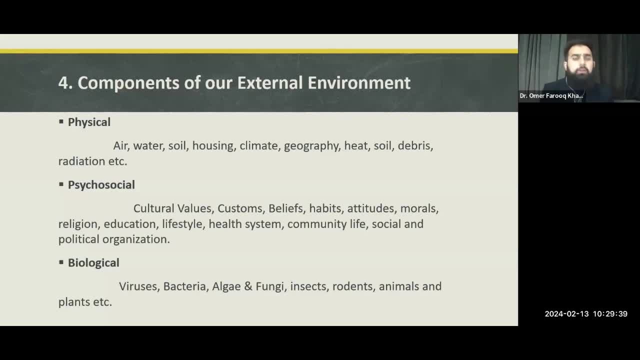 whether it's any kind of abiotic physical component or even biotech physical component. but if it is a physical component, it comes under the umbrella of this type of component. so air, water, soil, housing, climate, geography, soil debris, radiation, etc. and many more things, these uh constitute our physical uh environment. 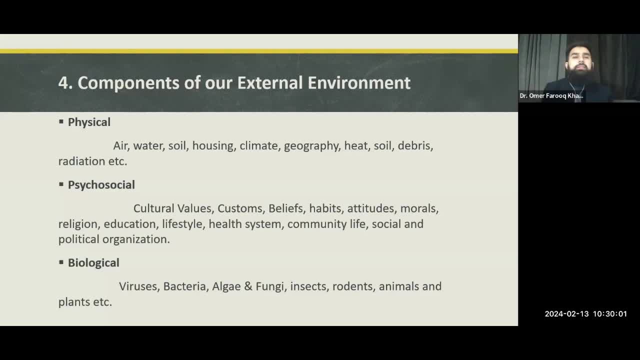 then there are psychosocial environment. so what is psychosocial environment? i already told that there are social sciences linked with environmental sciences. so our psychosocial environment plays a huge role in our mental health or our upbringing or our overall health. so psychosocial environment. 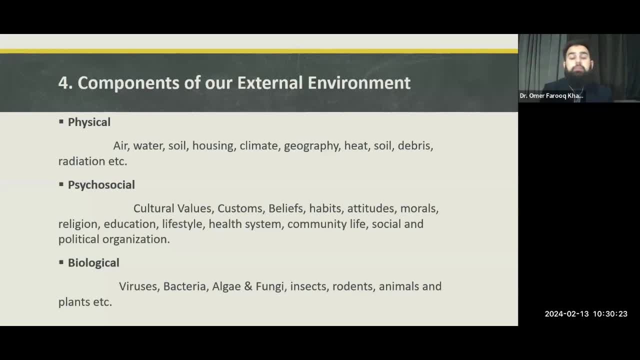 is also very important for us human beings, for example, cultural values, customs, beliefs, habits, attitude, morals, religion of any community, then the education of any community, then the overall lifestyle, then health system and all of these things. all of these things are very, very important. the psychosocial factors: 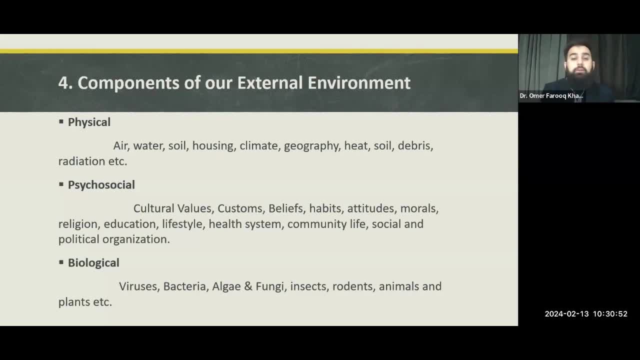 the psychosocial, uh component of our environment is very, very important, but so, uh, whatever the thought process runs in our mind is dictated by our cultural values. it is dictated by customs, beliefs, habits, attitudes, morals and our religion as well, then, how much educated our community is. 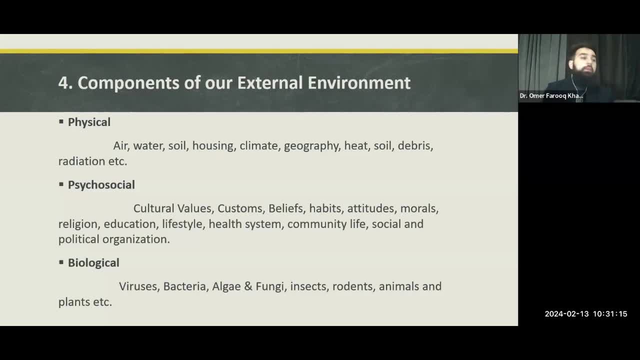 how what kind of lifestyles we have. there are communities which have very healthy lifestyles. people talk for kilometers daily, people are uh, sports loving, people are very energetic, people love to do exercises. and then there are communities where there is the hammy, where we're having a sedentary lifestyle is a norm, where people do not like to play much, where eating sugar or eating. 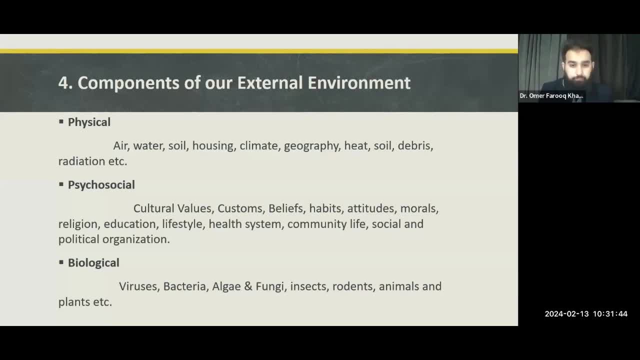 dairy products is a norm, and these kind of countries have very high rate of diabetes as well, very high rate of obesity as well. so lifestyles and education play a crucial role in our external environment. and then the health system. the health system dictates what kind of mortality rate is. 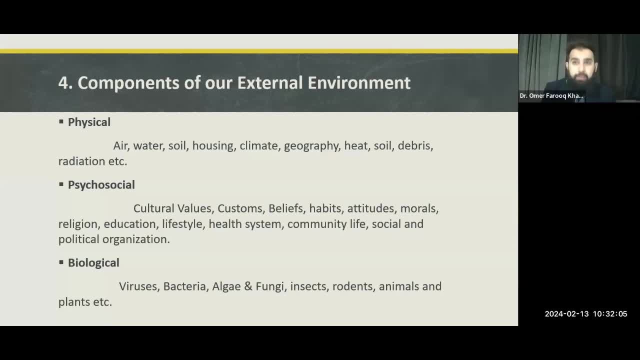 running in the community. what is the average age of any country is depicted by the quality of the health system. then there is community life, and then there is social and political organization of any uh country or any region. then there are biological components of our external environment. so 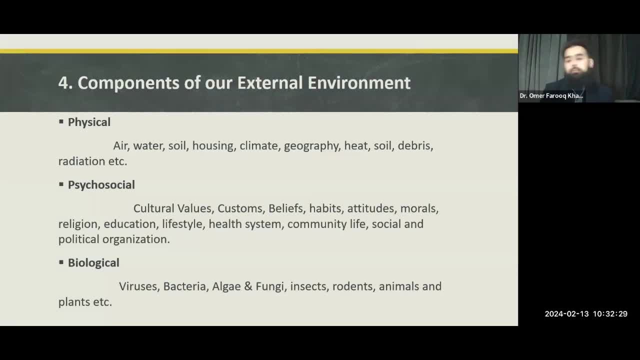 biological components, as the name depicts. you already know these are the living organisms in our external environment, for example, viruses, bacteria, algae, fungi, insects, rodents, animals and plants, etc. so any kind of living being which is present in our external environment is a living being which is in our external environment is a biological component of our external environment. 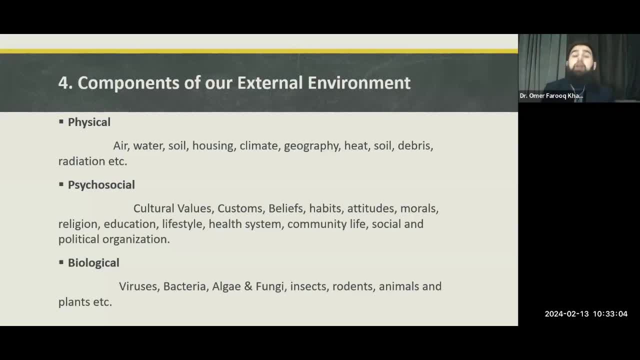 and biological component of our external environment also has a direct impact on our health. for example, in the case of covid, as we already know that there is a new virus and people are getting diseased with this new virus, and that new virus was in our communities and in our countries. then what happened? that tiny little microorganism which 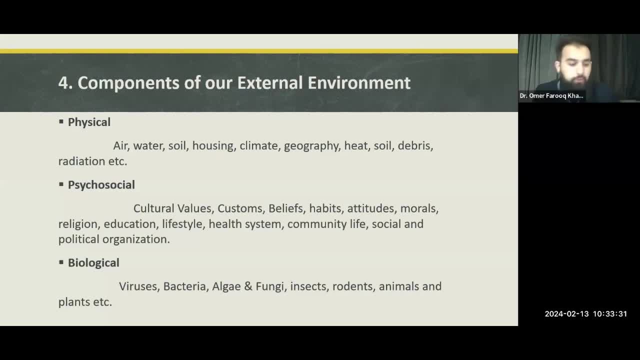 can't be even seen with any light microscope, it can only be seen with an electron microscope. but it govern the way we live for one or even more than one year all across the globe. so this one tiny little biological factor, or tiny little biological irritant of our external environment, 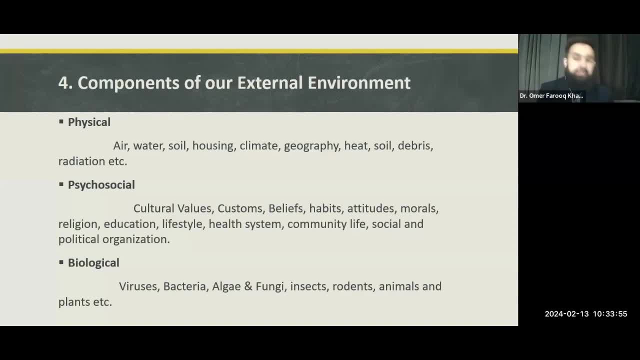 turned the world we lived in upside down. all of the flights were cancelled, all of the normal travel were cancelled, all of the hostling guidelines were cancelled. many people started getting dead from a simple flu-like illness and nobody knew what to do and nobody knew how to take care of. 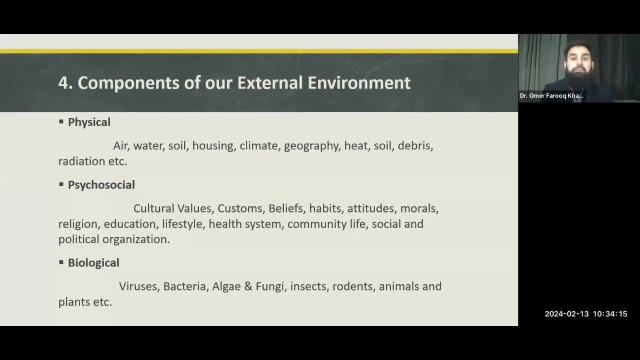 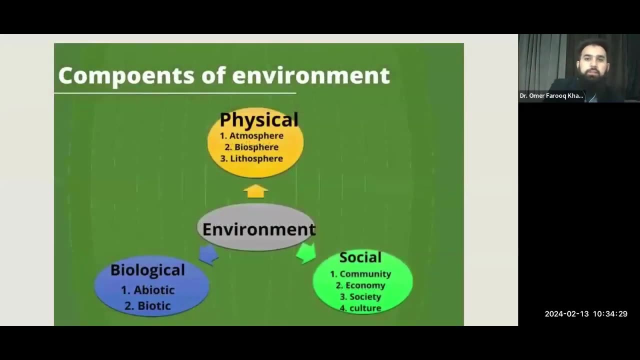 such patient, so even at times tiny little virus can have this much impact on our lives, then, and then we need to understand what bigger environmental factors have impacts on our human health and on our upcoming generation. so there is a diagram about the components of environment. so there are physical components. 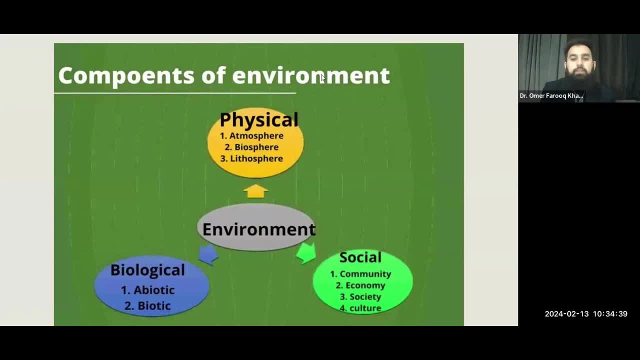 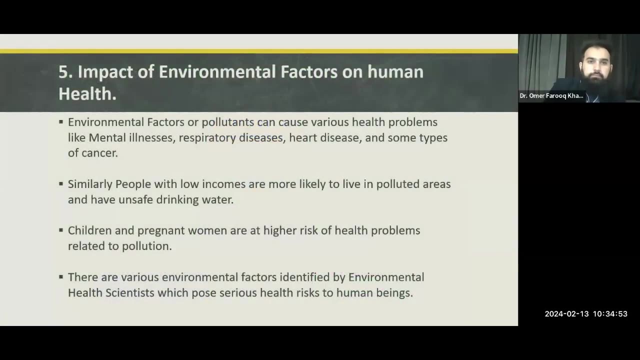 like atmosphere, biosphere, lithosphere. and then there are social components, as we already talked: community economy of the country, society, cultural norms, religion, education, political organization, that sort of. and then there are biological factors, such as abiotic or biotic. so in impact uh. now we come to talk about the big uh, the main uh subject of today's class, which is 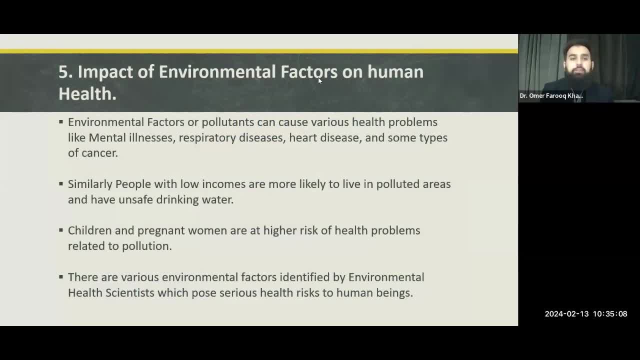 impact of environmental factors on human health. so environmental factors, or pollutants, can cause various health problems. drei health problems like mental illnesses, respiratory diseases, heart disease and sometimes of cancers as well. Similarly, people with low incomes are more likely to live in polluted areas and have unsafe drinking water. 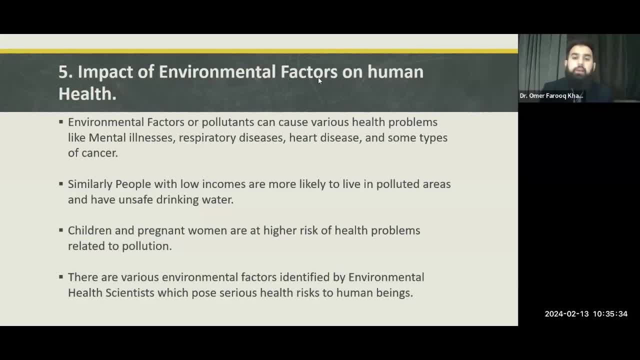 Children and pregnant women are at higher risk of health problems related to pollution. Then there are various environmental factors identified by environmental health scientists, which pose serious health risks to human beings. So any factor or pollutant which is present in our environment, in man-made environment. 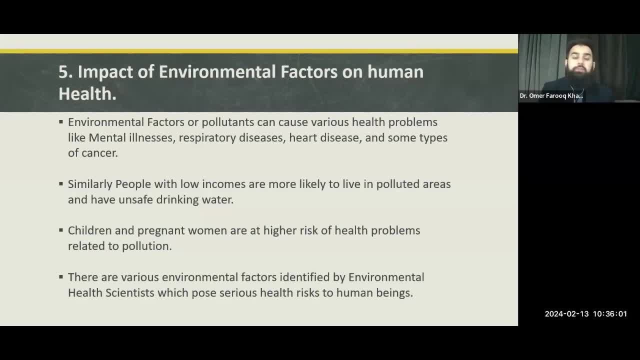 and it is causing health problems. it needs to be studied, It needs to be focused upon, It needs to be studied by us. It may be causing mental illnesses only. It may not be causing any kind of physical illness. It may not be causing any kind of physical illness. 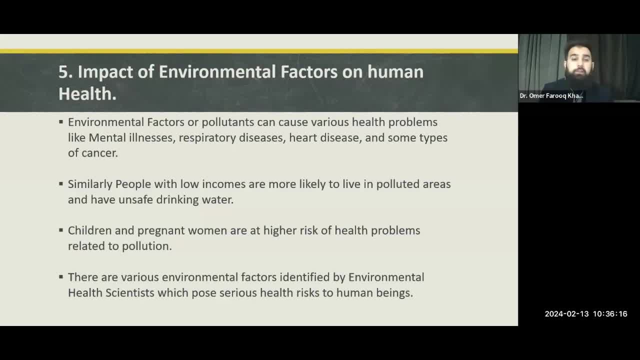 It may not be causing any kind of physical illness. It may be damaging the mental health of our patients only. It may only be damaging the respiratory diseases, It may only be damaging the heart diseases. It may only be causing the heart diseases And even it may be causing some types of cancer as well. 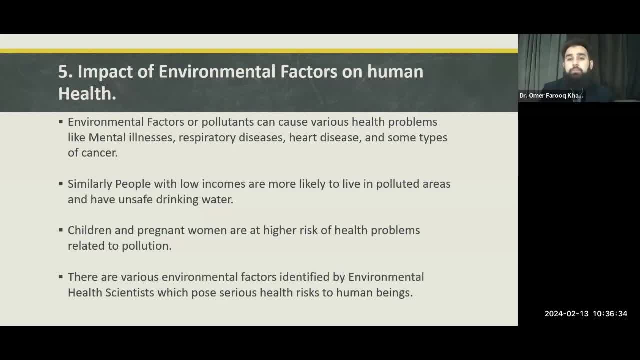 For example, in 1980s and 1990s it came out to be true that some scientists were skeptical about the use of asbestos, And then they came to know that asbestos causes lung cancer. The asbestosis causes lung cancer. 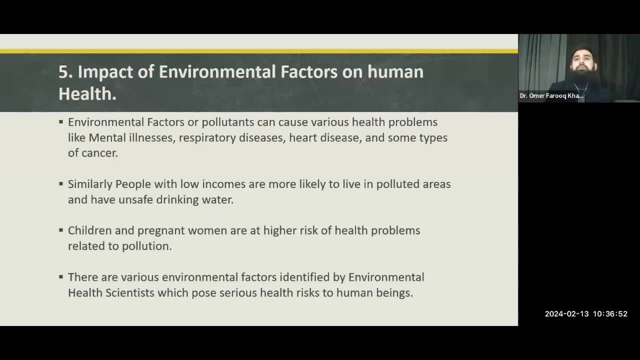 And then there was widespread ban on the use of asbestos in many industries. So if there was no research on environmental factors causing damage to the human health, the people would have been dying till date due to the factors which couldn't have been studied in the past. 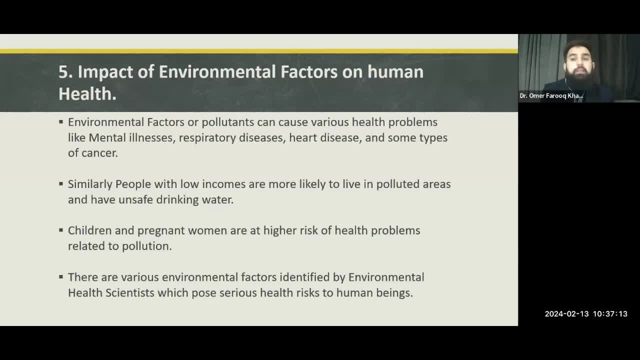 So it's just because of this environmental health That we have come this far, That we have come to know that many of the things which were considered safe for human consumption or which were considered safe for human contact, are not considered safe anymore, And those things are now brought back from the natural industry. 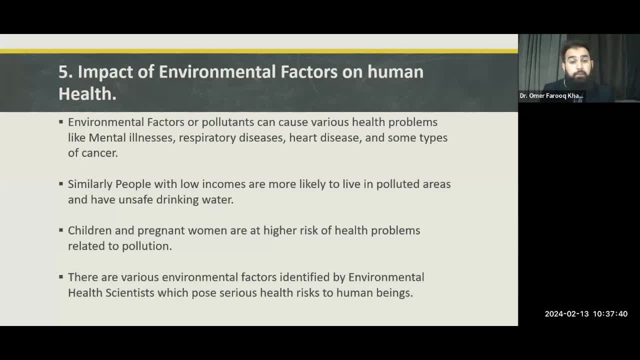 Similarly, the low income problem, Which is Present in many countries, is also a problem. So if a country has low income, then their health system is fractured, Then their nutritional system is fractured. So all of these people, All of these people whose health system or nutritional system is fractured, 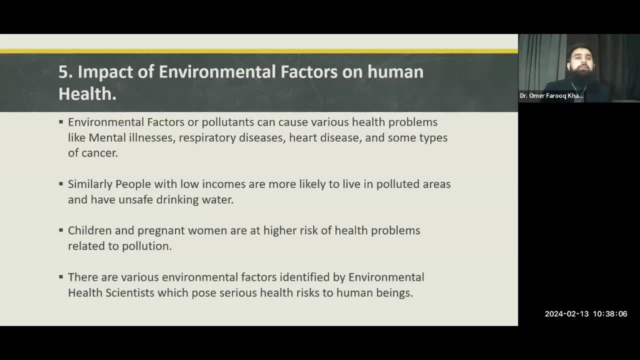 They are likely to get more diseases related to the poor nutrition. So their environmental factors are causing diseases. So their environmental factors are causing diseases In such people And similarly, as we already know, children and pregnant women are at higher risk of health problems related to pollution. 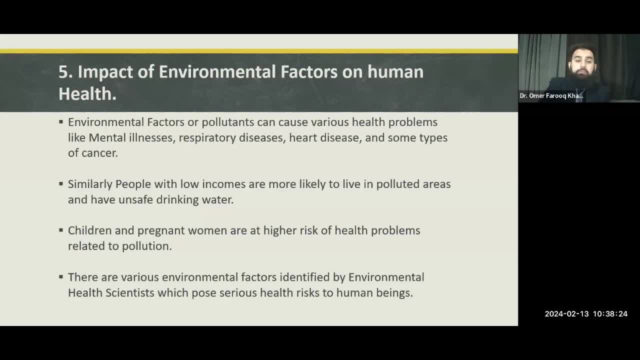 Children and pregnant women are the vulnerable section of the society, Even, I should add, the elderly as well. So children, pregnant women and elderly are at higher risk of health problems related to pollution. There are various environmental factors identified by environmental health sciences which pose serious health risks to human beings. 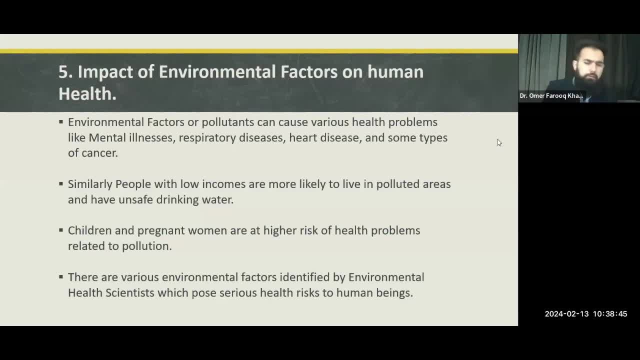 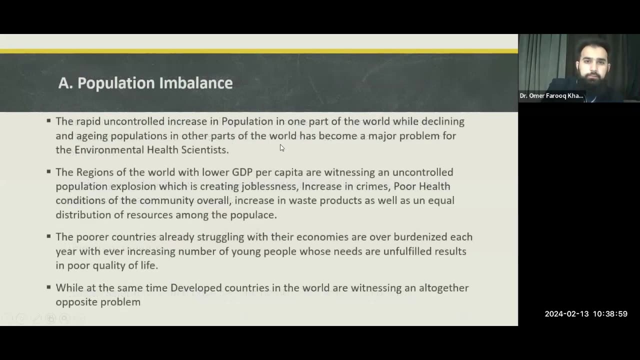 And this is a Very broad subject. There are many environmental factors. I will focus on three environmental factors which have direct impact on human health in this class, In today's class. So the first environmental factor having a direct impact on human health is population imbalance. 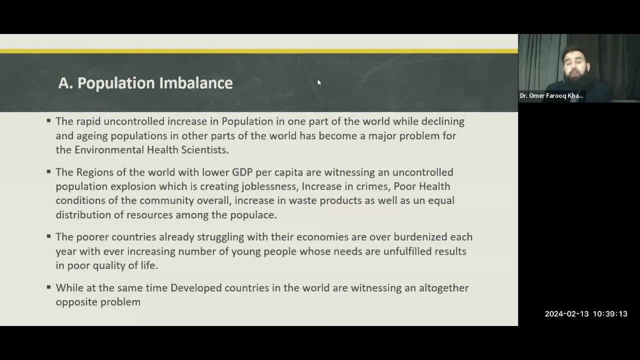 So I don't. I did not use the word population explosion as, As per my research, there is this: This term is not correct And by this term is not correct. I will defend that viewpoint in my evidence as well. So I use the word population imbalance instead of population explosion. 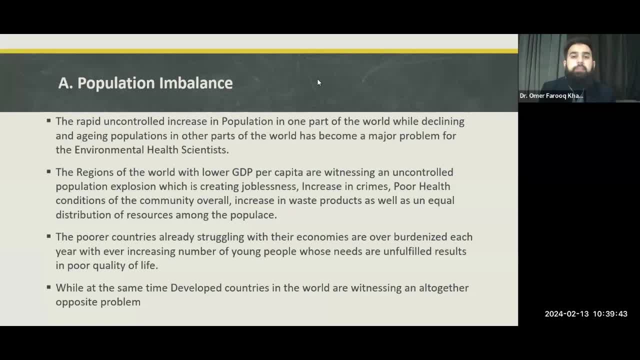 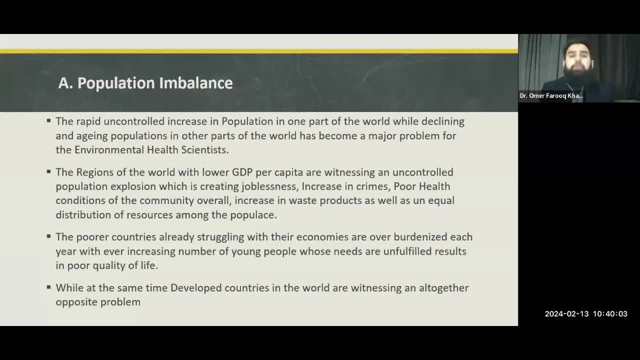 So the rapid Uncontrolled increase in population in one part of the world, while declining and aging populations at the same time in other parts of the world. The rapid uncontrolled has become a major problem for environmental health scientists. Similarly, the regions of the world with lower GDP per capita. 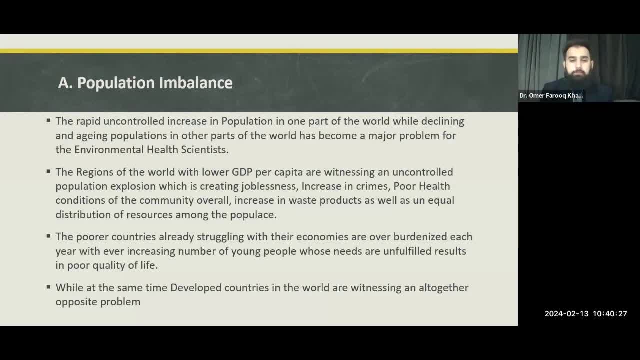 are witnessing an uncontrolled population explosion which is creating joblessness, increase in crime, poor health conditions of the community, overall increase in waste products, as well as unequal distribution of resources among the population. So the problem with the population imbalance is. 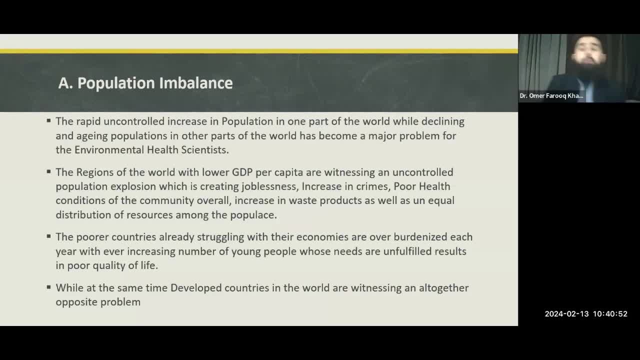 those countries which cannot carry the burden of already existing populations are adding to their population at a much faster rate than they can carry on. They are already under debt. Those regions or those countries are already under too much stress of joblessness, So the joblessness rate in such countries is already very high. 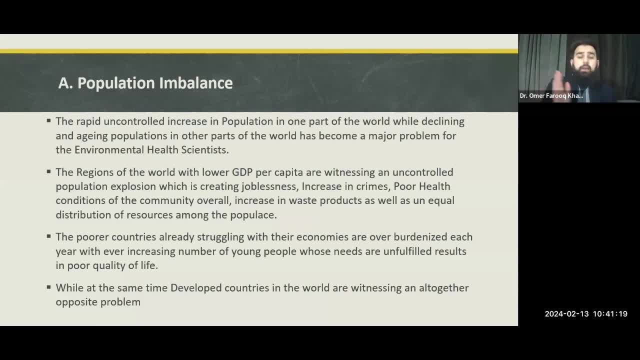 Crime rates are already skyrocketing. Health conditions are already poor. The problem with the waste products. too many waste products in the air, water or soil are already there And still they are unable to control their booming population And they are already unable to feed their present population. 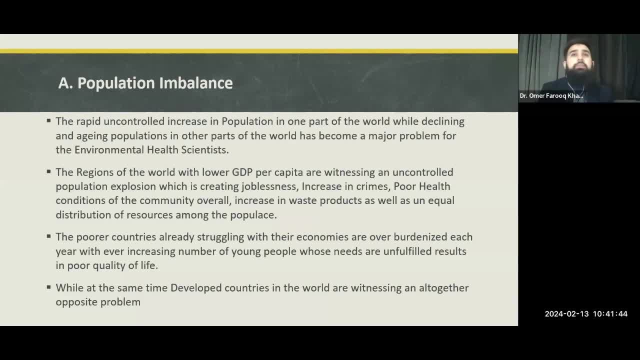 But the future population of those regions is increasing at a much faster rate, at an unsustainable rate, And the poorer countries, already struggling with their economies, are overburdenized each passing year with ever increasing number of younger people whose needs are unfulfilled, resulting in poor quality of life. 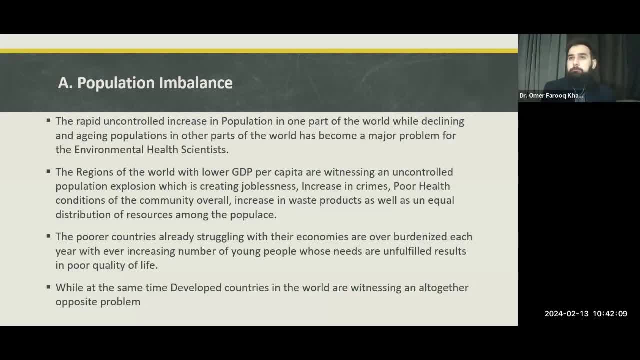 So basically any country, for example, I will talk about uh, any uh country A. I will not name any country because that might offend some people here. So I will not name any country. For example, any country X, Y, Z. 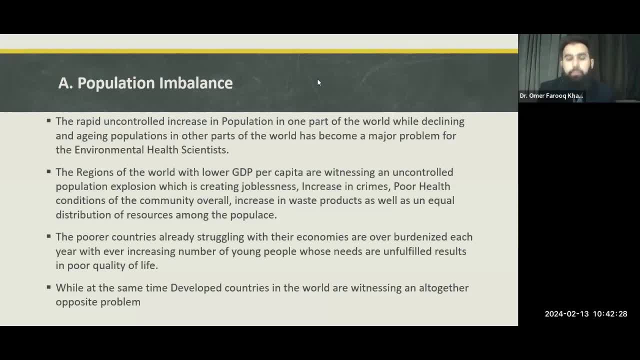 whatever that country is, is already under debt, is already struggling with poor health conditions, is already struggling with the joblessness crisis, is already struggling with the increasing crime And there is overburden, and that country is also overburdened each year. 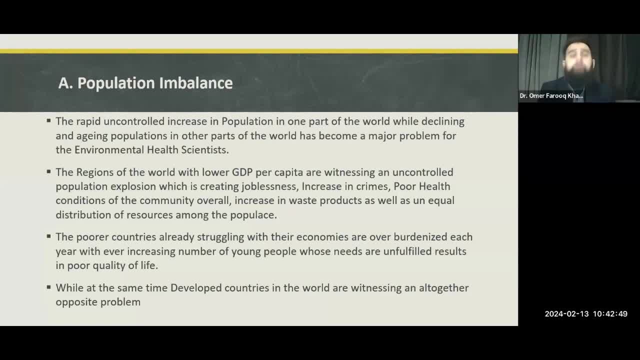 with ever increasing number of young people whose needs are unfulfilled. It creates a disaster, It creates a problem And, at the same time, when we are talking about the poorer countries, creating too many young people, creating too many population, at the same time. 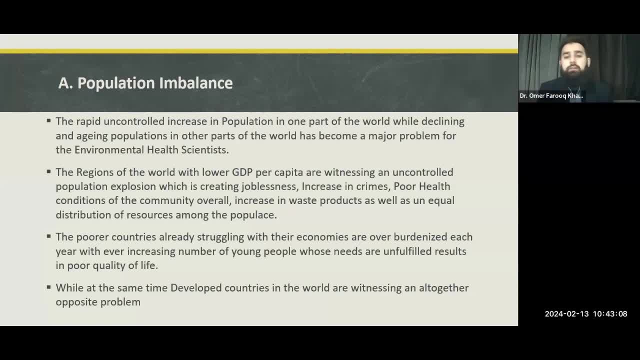 the developed countries in the world are witnessing an altogether opposite problem. So the developing world, the poor world, is creating too many humans whose needs are unfulfilled more than ever, And then, at the same time, the developed countries in the world. 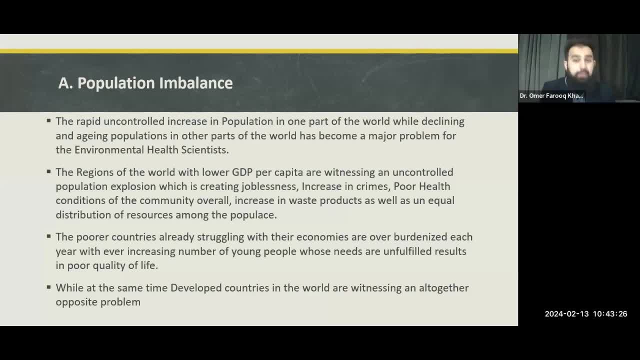 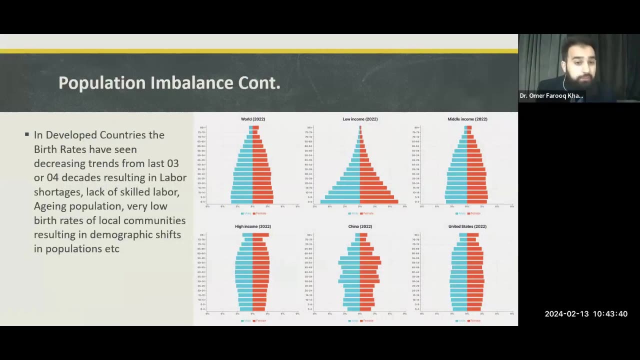 who can sustain the increasing population are witnessing an altogether opposite problem, And what that problem is. in developed countries, the birth rates have seen decreasing trends from the last three or four decades, resulting in labor shortages, lack of skilled labor, aging population. 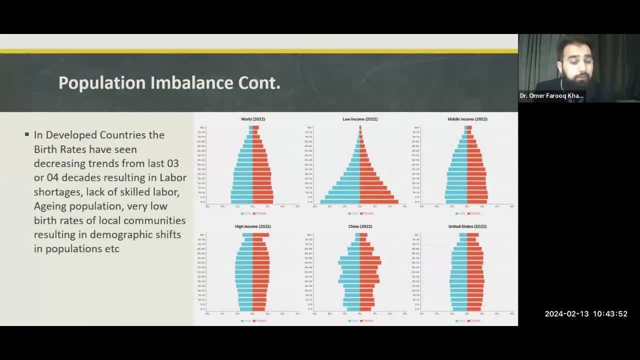 with very low birth rates of local communities, resulting in demographic shifts in populations as well, So this is not a population explosion problem. I know many people will talk about the aspect that the poor countries, that the poor countries are more and overall the world is increasing its population. 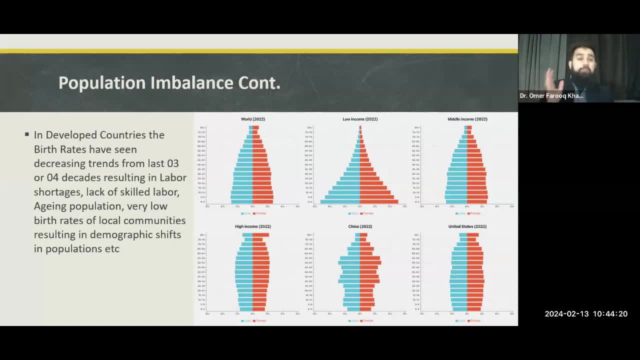 et cetera, et cetera. But there are many, many countries in the world which are considered as developed countries and these countries are having an altogether different problem, For example if we talk about the population parameters. So here in this slide I added population parameters. 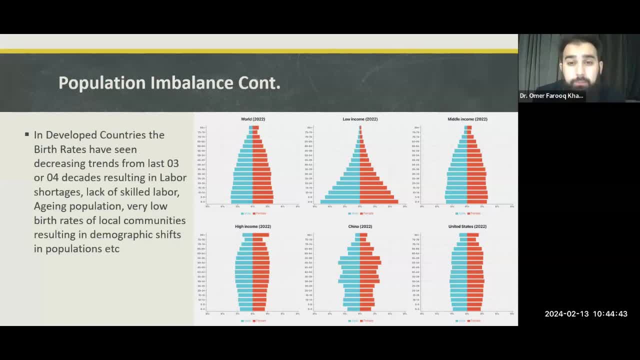 So here in this slide I added population parameters. So here in this slide I added population parameters. So these population parameters are very easy to understand. So these population parameters are very easy to understand. So these population parameters are very easy to understand. 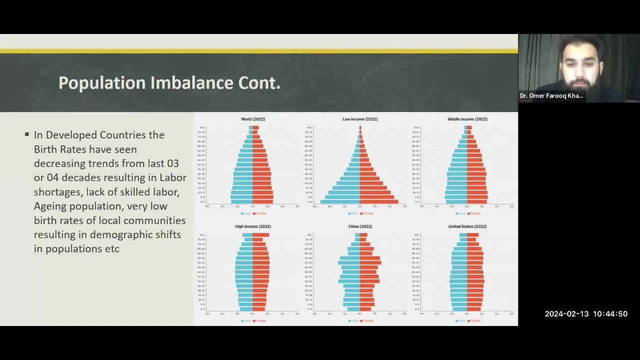 I know that mentioning these parameters, maybe composers already know the population parameters On this slide. it is a geographical presentation of people of different age groups and their percentage in the total population. So if you click cart, For example, the word gives a scientific concept based inロ suspect. 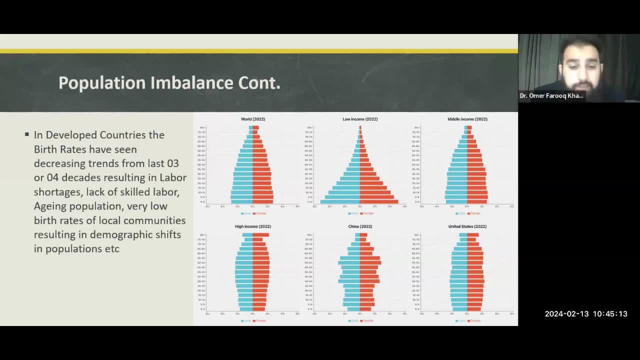 a mixed picture. more of the world contains of younger population, as we are already seeing in the 2022 data, but at the same time, what is happening in the low-income group of the world? what is happening in the low-income countries? the low-income countries are over burdenized with 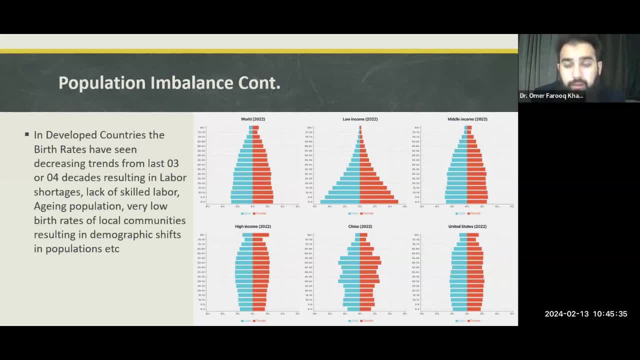 too many young people and they're already struggling with the joblessness problem. they're already struggling with poor health conditions. they're already struggling with the poor education system. they're already struggling with very primitive industrial base, but at the same time, their growth rate is increasing at a much faster rate. 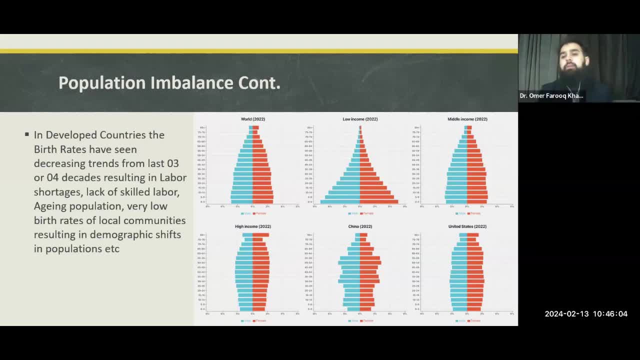 than the rate they can sustain. and then there are middle-income countries. the middle-income countries also give a mixed picture, but their overall are also. but these countries are also moving towards positive growth, balance positive growth, positive population replacements- as the popular, positive growth is like the people. 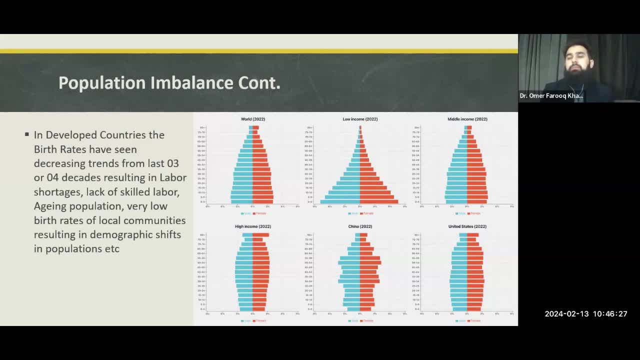 dying per annum are less than people being born per annum. then there is a high income group, for example. for example, just the test case scenario- we talk about germany. so germany has a problem that the germany and japan- there are two, two countries- these countries have a problem of aging. 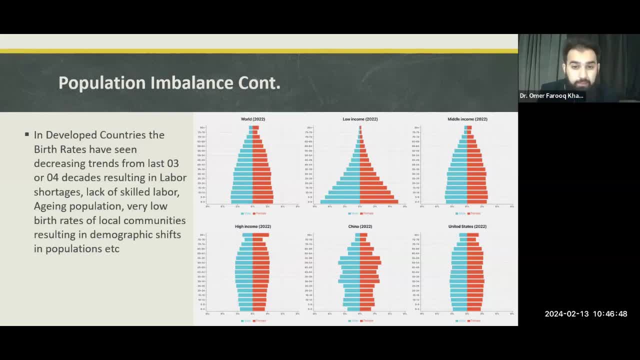 populations. now look at a high income country and the problem with the high income countries: the zero to four and five to nine age group is shrinking, but the middle age and higher age groups are getting wider. so basically what is happening, the uh, the phenomena here, is that more. 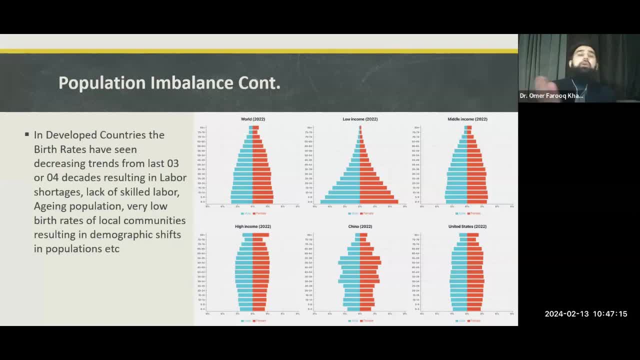 and more people. even they are rich. even they can afford to have healthy babies. even they afford to give them health, very good education. even they can afford to give them very good health condition. even they can afford to give them all the needs of the world. but they have chosen. 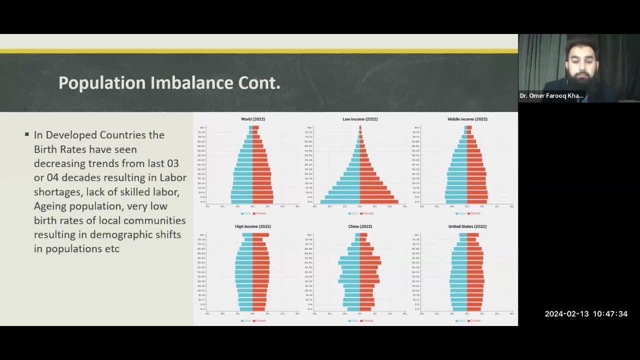 not to have kids. so what is happening in high income countries? those kids which should have been are which, which are in a very higher number in low-income countries, are here here. their strength is getting low. here. aging population is greater than the replacement population. the young kids being born are less. 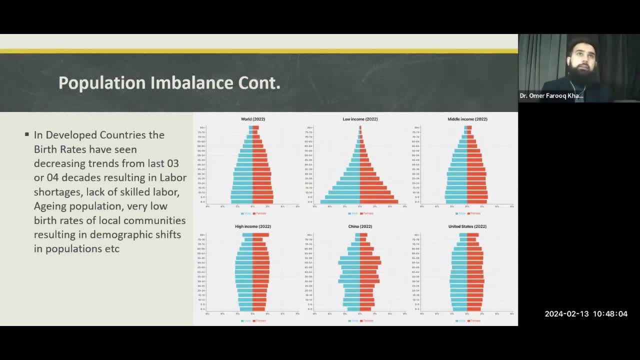 and the people getting old and the people getting the people dying are more what's happening. what's the problem? these countries have very good industrial base. these countries have very developed health system. these countries are very, very developed education systems, but the problems which they are suffering from is that their industries. 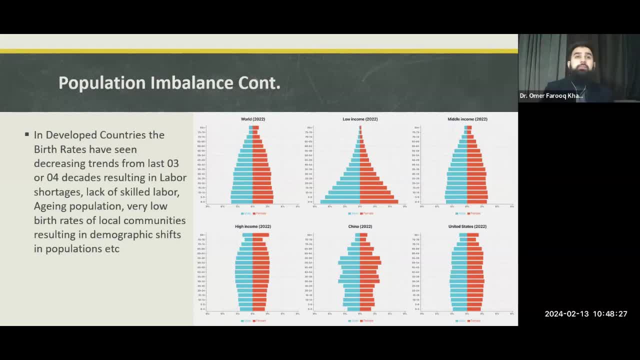 are are having severe labor shortages. they have a grown industry, they have built up industry, but there is no skilled labor to run that industry because their population is in negative. they have no younger people coming in to replace those people who are getting old. there are no younger people coming. 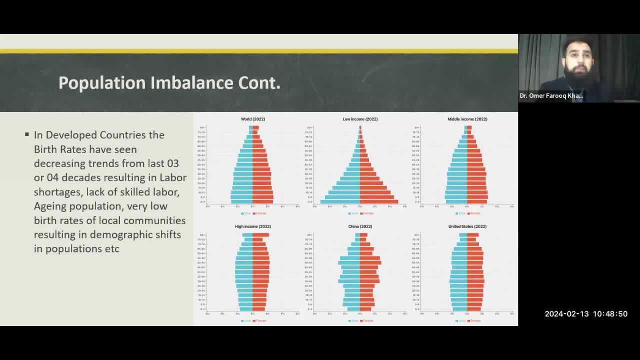 in to replace those people of the middle middle age group who are getting retirement. so the problem is they have to import the skilled labor from the low income or middle income countries, for example. i will give example of my own country, pakistan, for example. i will give example of my own country, pakistan. so we 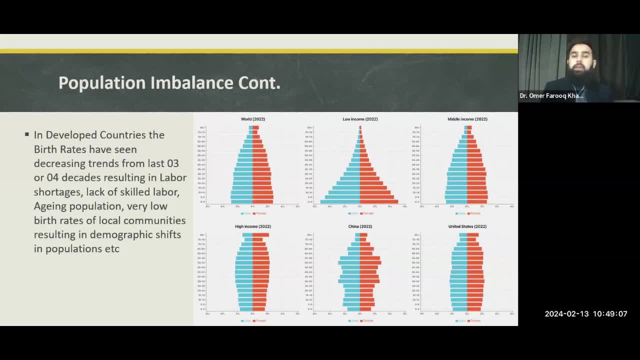 export. so we export too much skilled labor every year. too much skilled labor every year, in this year alone, in 2023, in past year, in in this year alone, in 2023, in past year, in past year alone in 2023, in past year alone in 2023- one million. 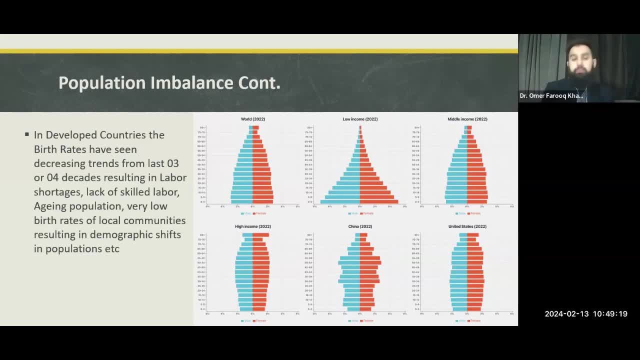 one million skilled labor was exported to high skilled labor was exported to high income country, income country. and why? because the high income country. and why? because the high income country grow. its own population is shrinking. they have a. its own population is shrinking. they have a developed industry, but there are no people to run that industry. they are. 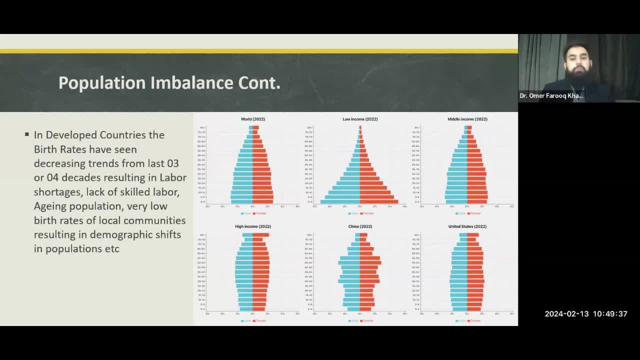 developed industry, but there are no people to run that industry. they are developed health, education, health system and education system, but there are no people to run that health system and education system. similarly, in the case of china, the growth rate of younger population has decreased drastically and now they are worried. they had a one child policy for 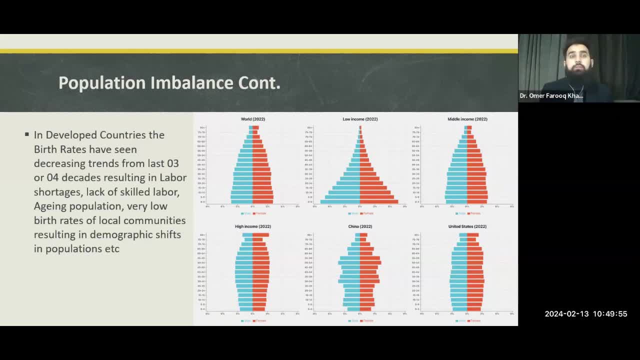 almost four decades, for decades, and now they are worried that their policy has backfired and they are getting, they are suffering the from the problem of the same rich countries, and the problem is people are not having more kids and their industry has increased drastically. their industrial 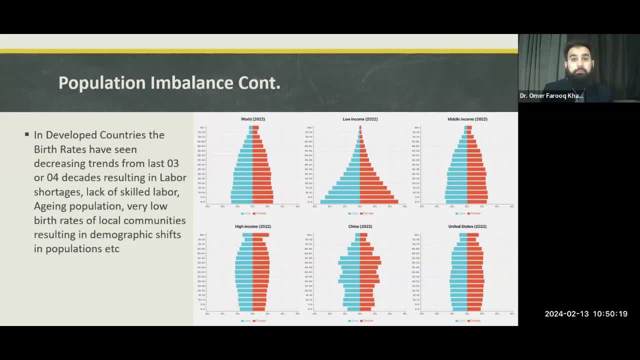 basis widened drastically. but now the problem is they are also suffering. i'm talking about china. they are also suffering labor shortages. they are also suffering from the lack of skilled labor. it's just you, you, just because of this population, mismanagement on behalf of the government. similar is the case. 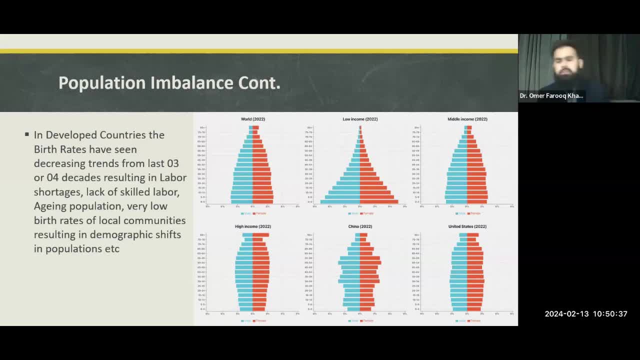 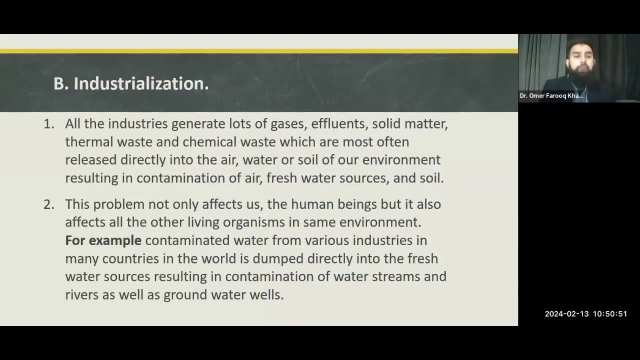 with the united states, but united states is a slow growth country where the people dying are still less than people being born. i hope you people got what i try to deliver. then there is a second environmental factor, a very important environmental factor, and that is industrialization. so all the industries generate lots. 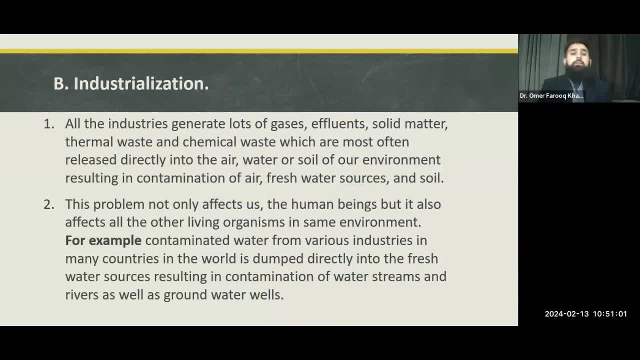 of gases, affluence, solid matter, thermal waste, chemical waste- which are most often released directly into the air, water or soil of our environment, resulting in contamination of air, fresh water sources as well as soil. so it used to happen. if we go back 40 or 50 years back, the laws were very lax. there was no regulation, regulatory bodies. there was no. 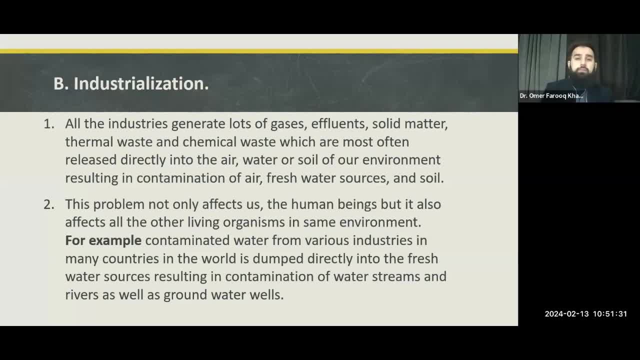 proper system. even in today's world, in developing countries or in poor countries, there are no laws which govern any kind of industries, because there are already very less industries and they want people to invest in their country and they do not want the industries to run away from their countries. 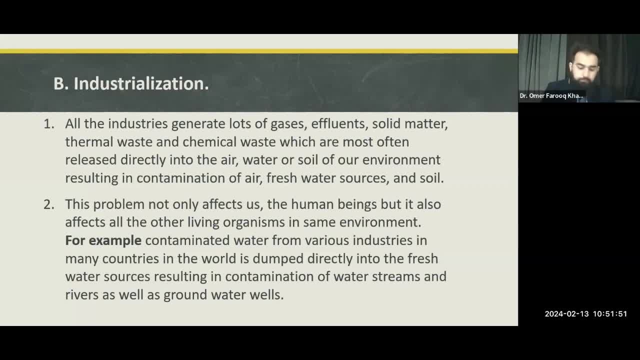 due to lawlessness, due to crime rates, due to militias harassing them. so there are already countries which have very lax laws, which are very lax laws, which are already very lax laws, which are who do not question the industries about their waste products, But there are countries which are already taking care of industries. 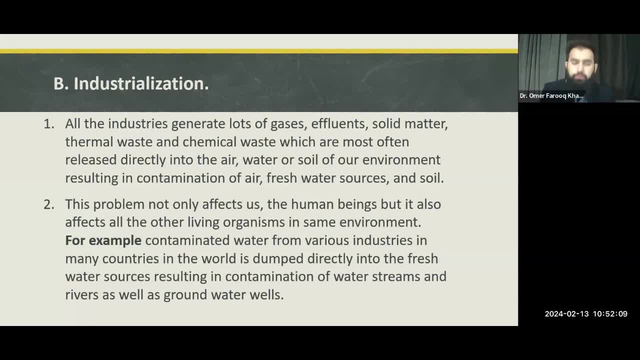 so that their waste products can be controlled. But overall, if we talk about the whole of the planet Earth, the industries generate lots of waste products which are hazardous to human health, And this problem not only affects us, the human beings, but it also affects all the other living organisms in the same environment. 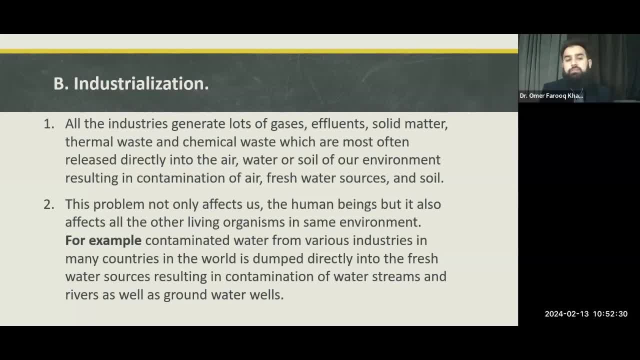 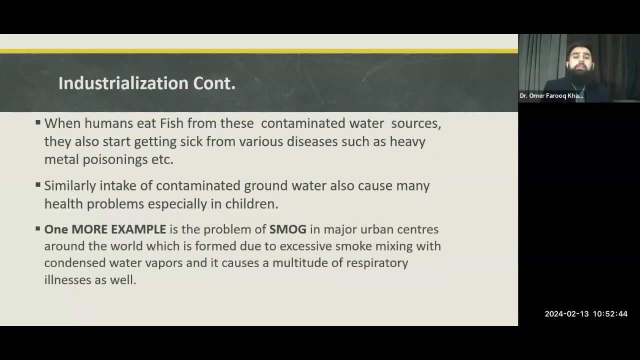 For example, contaminated water from various industries in many countries in the world is dumped directly into the fresh water source, resulting in contamination of water streams and rivers, as well as groundwater wells. When humans eat fish from these contaminated water sources, they also start getting sick from various diseases, such as heavy metal poisonings, etc. 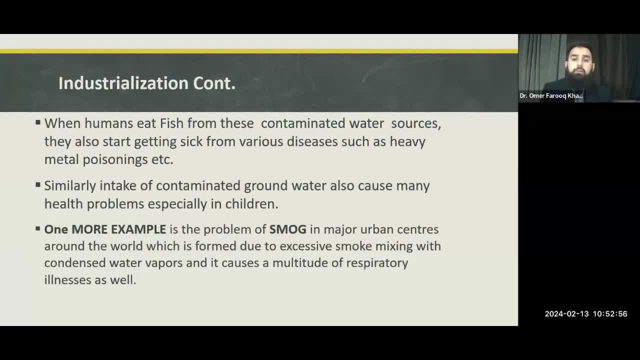 Similarly, intake of contaminated groundwater also causes the environment to be polluted. This also causes many health problems, especially in children. So it's just like the old saying: what you sow, so shall you reap. So whatever damage we cause to our environment, 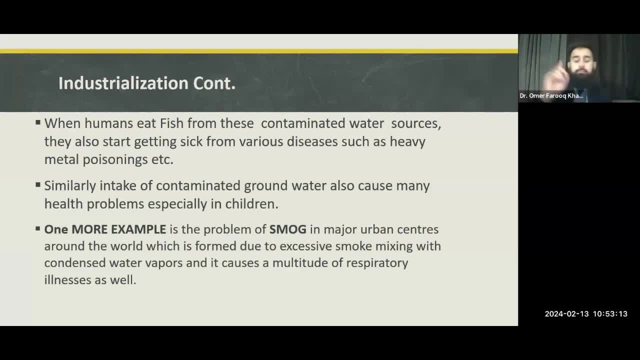 it reflects back on our health because of the deterioration of our external environment. One more example is the problem of smoke in major urban centers around the world, which is formed due to excessive smoke from contamination of water, So the pollution from the pavement. 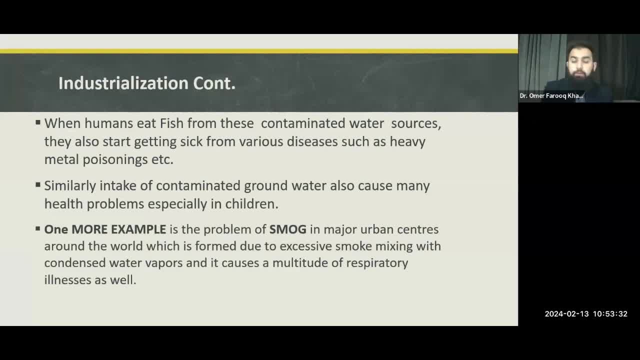 the pollution from the combustion engines, excessive smoke from industries, excessive smoke from rotary kilns mixing with condensed water vapor, and it causes a multitude of respiratory illnesses as well. So I gave you two examples. One is the contaminated water from the industries. 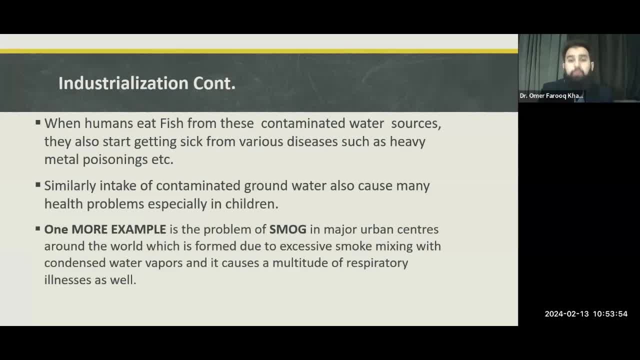 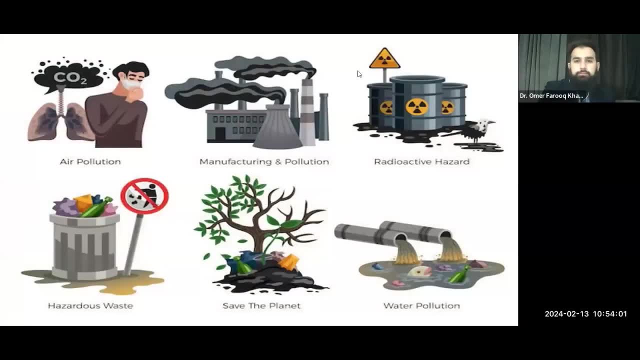 and then there is the example of smoke which is caused due to the industries. So the pollution causes also many respiratory illnesses and it causes even more respiratory illnesses gases. so all of these things are having very much, very problematic, hazardous effects on human health. so air pollution here is causing many kinds of 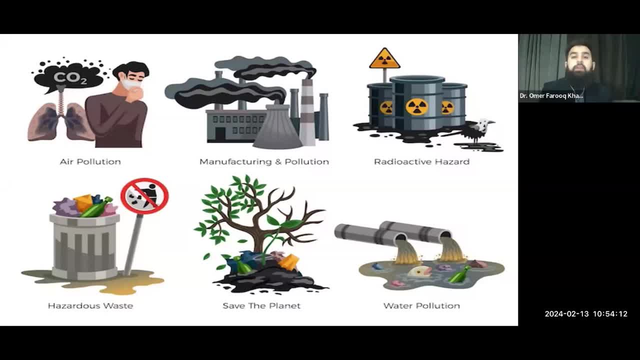 respiratory illnesses. then there is manufacturing and pollution. many manufacturing units create too many hazardous synthetic chemicals which are left untreated into the surrounding environments, rivers or soils, etc. then there are radioactive hazards related with the nuclear activity. then there is hazardous waste which is hazardous for the kids and overall community as well. 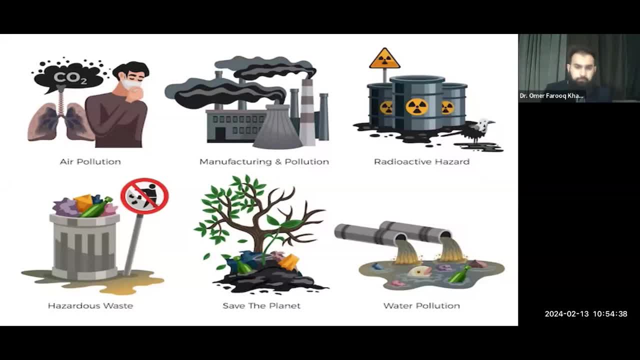 then there is plastic problem, which is causing deterioration of all of the green lands of the planet. then there is water pollution. water pollution as the untreated water is directly dumped into the fresh water sources of the community, and when the community uses that polluted fresh water, all of the community, including human beings as 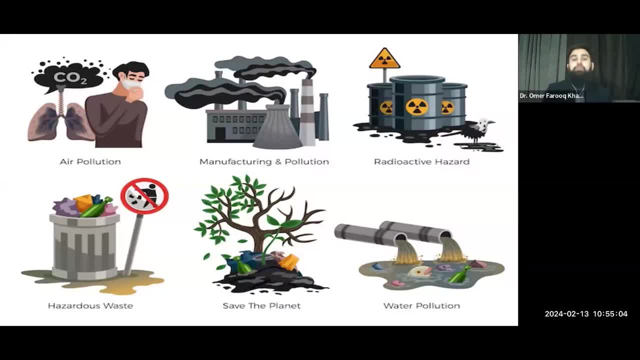 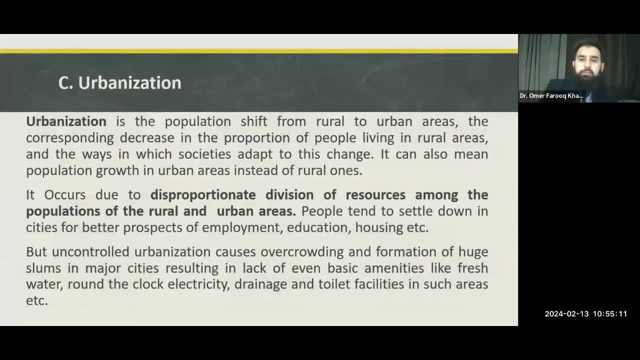 well as animals and plants, gets affected due to the use of that polluted water, starting from the fish. then the third problem with our environment, which environmental factor affects our health, is urbanization. it's the last thing. I will try to wind it up as early as possible so we can take maximum questions as well. 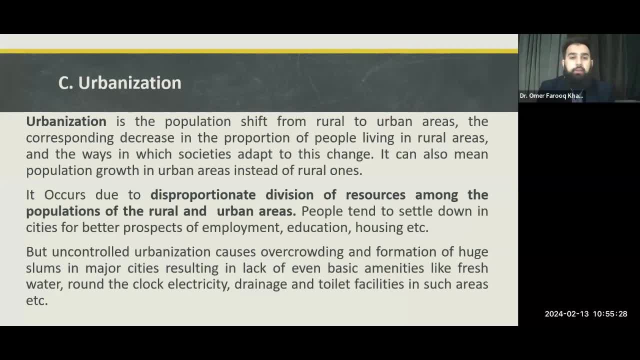 if you have any background, what do you think we should talk about? first i will take a second question, all right guys. then I show you what are the common problems that we face in this new era and then I will make them Crossführer. massive affected by urbanization. 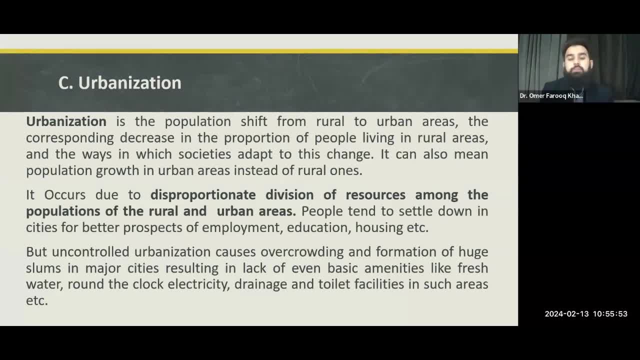 urbanization is a population shift from rural to urban areas, the corresponding decrease in the proportion of people living in rural areas and the ways in which societies adapt this change. it can also mean population growth- urban areas, due to which people in the need of or in the pursuit of better resources start moving. 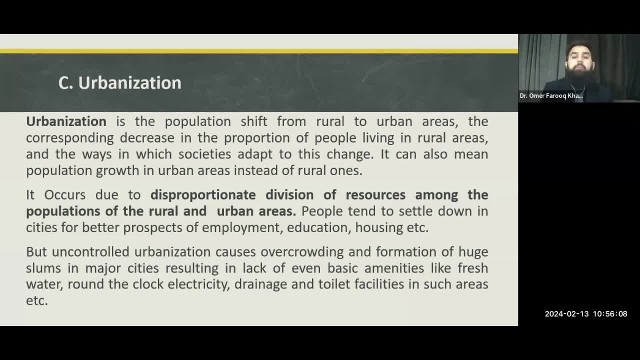 towards the cities. people tend to settle down in cities for better prospects of employment, education, housing, etc. but uncontrolled urbanization causes overcrowding and formation of huge slums in major cities, resulting in lack of even basic amenities like fresh water, round-the-clock electricity, proper drainage system and toilet facilities in such areas as well. 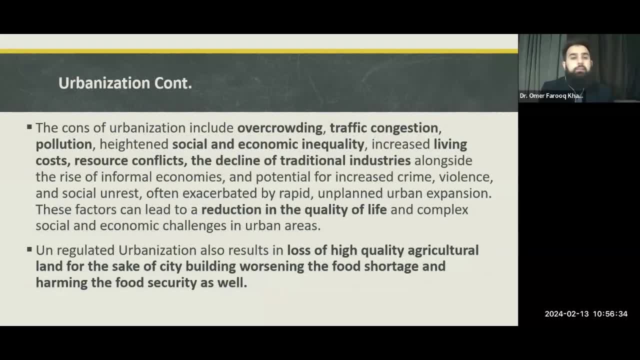 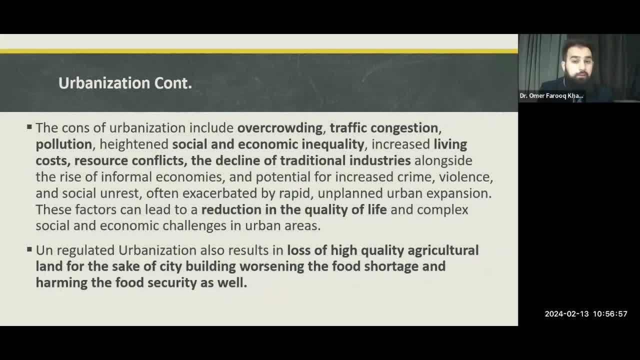 industries, alongside the rise of informal economies and potential for increased crime, violence and social unrest. often exacerbated by rapid, unplanned urban expansion. these factors can lead to a reduction in the quality of life and complex social and economic challenge in the urban area. so unregulated urbanization. 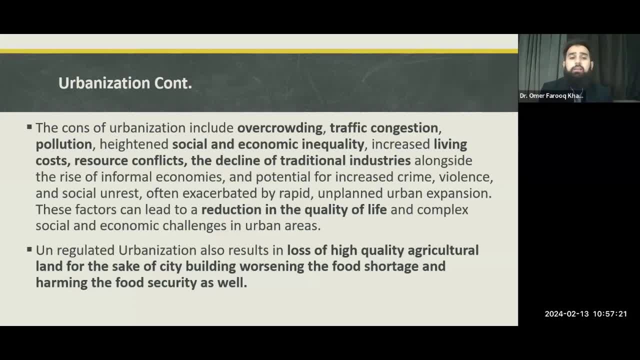 also results in loss of high quality agricultural land for the sake of city building. this phenomena is worse in our in my country, pakistan. so there are too many housing societies being built on agricultural land and the government does nothing about that. if the government start or wants to do, 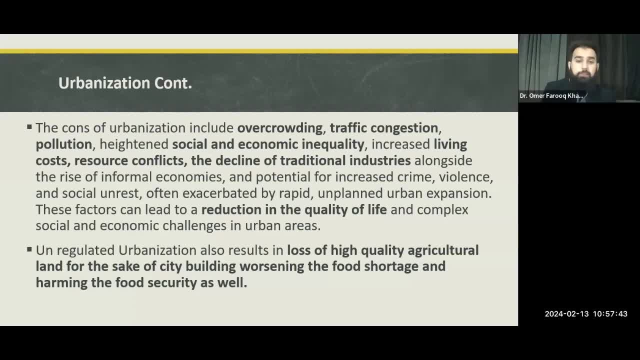 something about that. the mafia- the real estate mafia, the builders mafia- just sabotages the political business and the government does nothing about that. so unregulated urbanization and the politicians get blackmailed for the lack of sport or they are blackmailed due to many other. 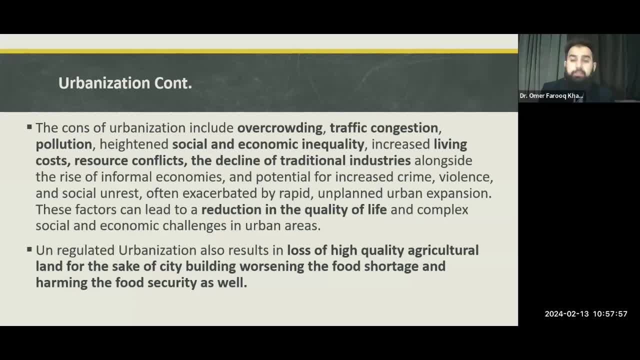 reasons, or even they are bribed not to pass laws against the housing society's illegal housing societies or illegal housing projects. so if there are no laws and if there are very lax laws, the agricultural land gets destroyed for the sake of city building, worsening the food shortage. 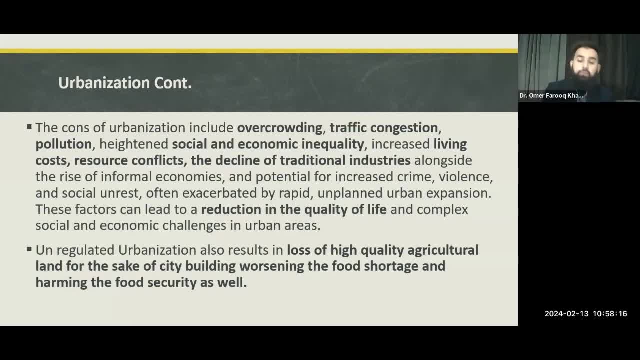 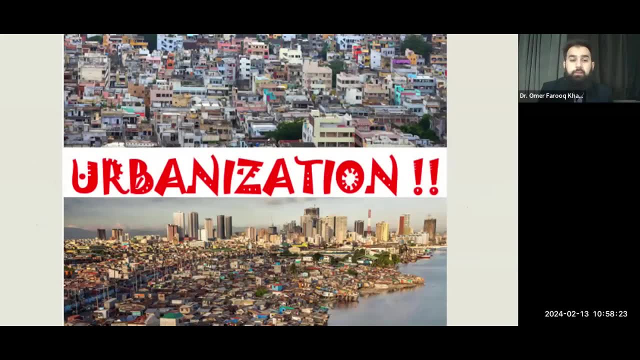 already present in such countries and harming the food security of such countries. so unregulated urbanization also get us in trouble as well. so this, this picture depicts uncontrolled urbanization. if you look at above picture, it is a haphazard growth of a city with no proper street.